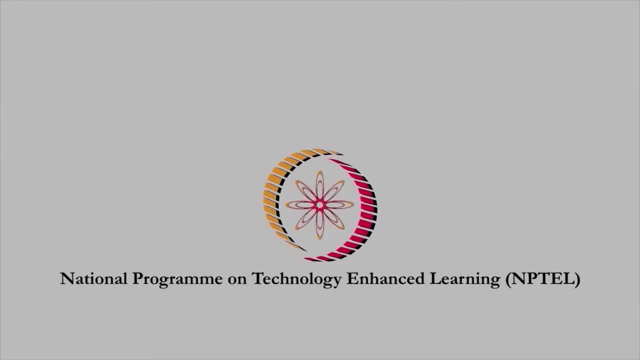 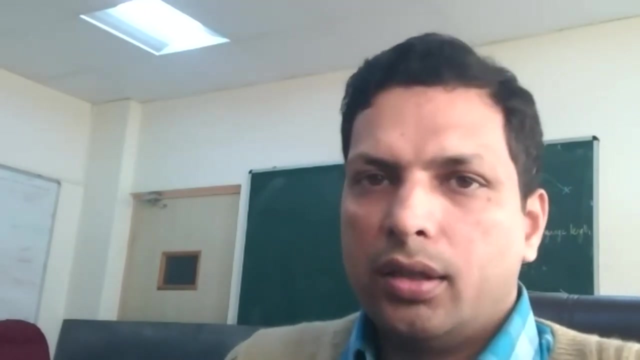 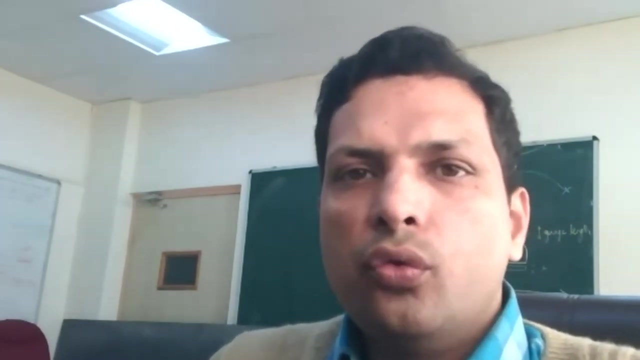 Welcome back students. We have looked at the dislocation characteristics, We have also looked at dislocation motion and we also looked at the fundamentals which define the slip system. So on what particular plane in a given material system would the dislocations move? Next we are going to look into a very important concept related to dislocations. 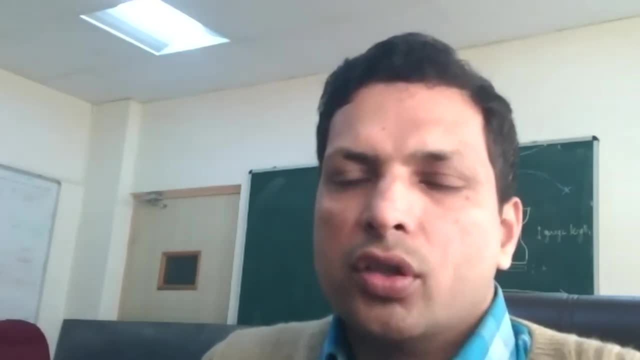 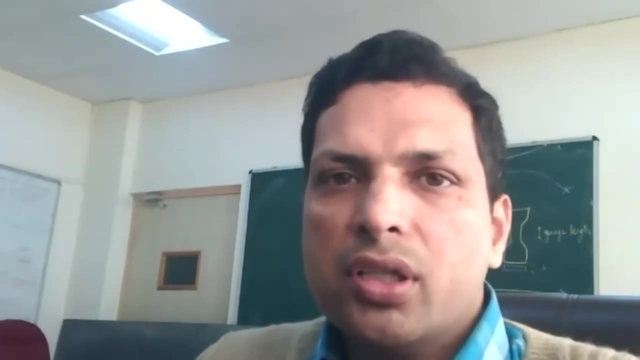 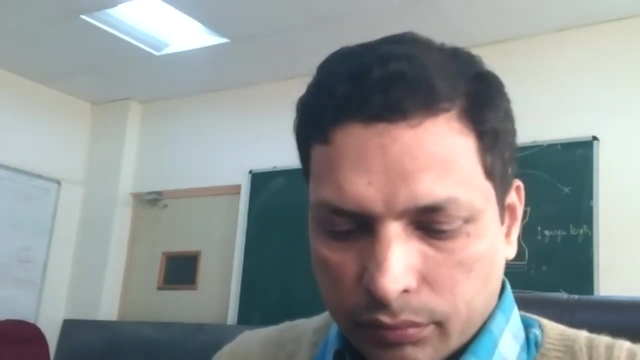 which is critical, resolved shear stress, which is what defines how much or not defines, but this is what will help us determine what will be the stress required for dislocations to move. So let us look into it. Let us assume we have a single crystal, So this single 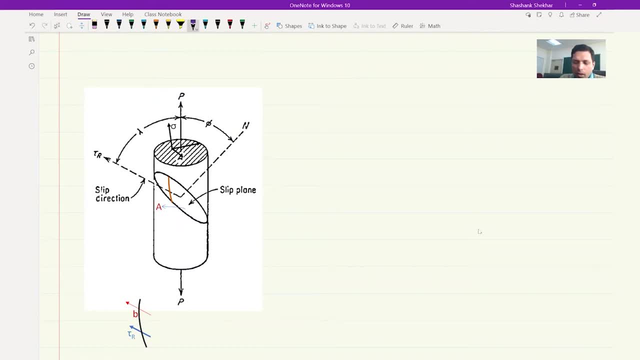 crystal is in the shape of a cylinder like this, and inside this we are looking at one particular slip plane. So the question we are asking is how much stress or load we need to apply, say along P. So P is the load here, and if you know the area then we know what stress is to be. 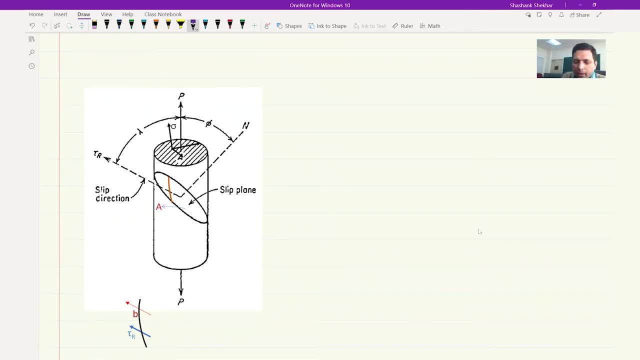 applied. So sigma, you can say, is to be applied in this direction for the dislocation to move. We know that the dislocations will move only under shear stresses. So the question is, what will be the resolved shear stress along the Berger vector? So let us say, if we were looking at dislocation 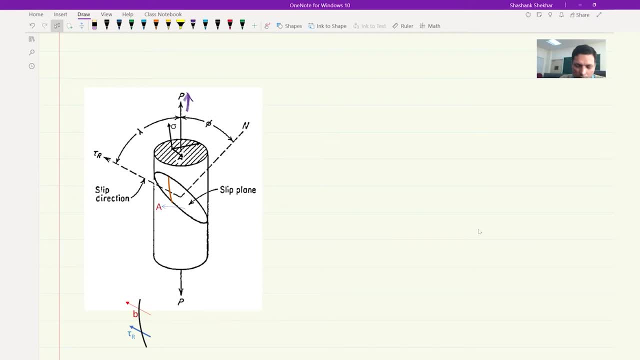 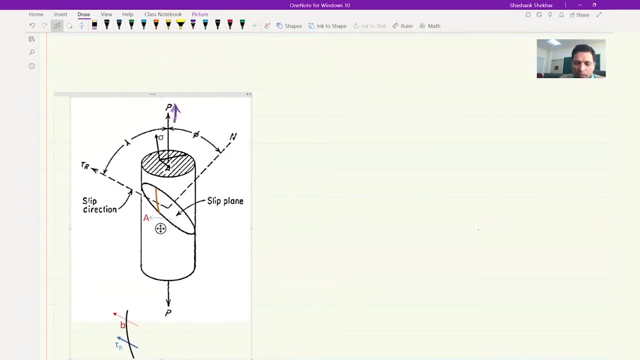 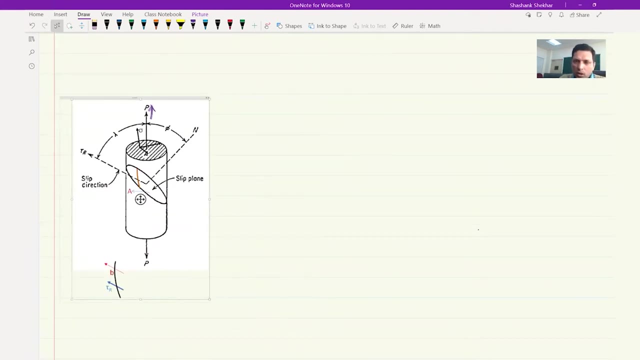 independently, which is shown in the bottom here, and this is the Berger's vector. then what we are interested is in finding that what will be the total shear stress acting along Berger's vector and on the plane on which this dislocation can move? So this: 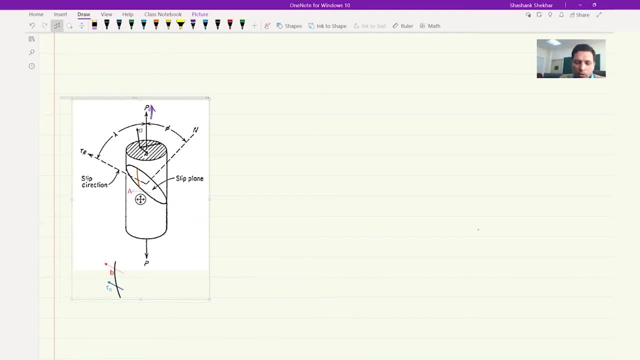 is what we want to identify and it has to. and here we have given the load in terms of P and we know the area A, or you can have as well defined it in terms of sigma. So let us say we want to find out the stress, So that way we will know what is the stress required. 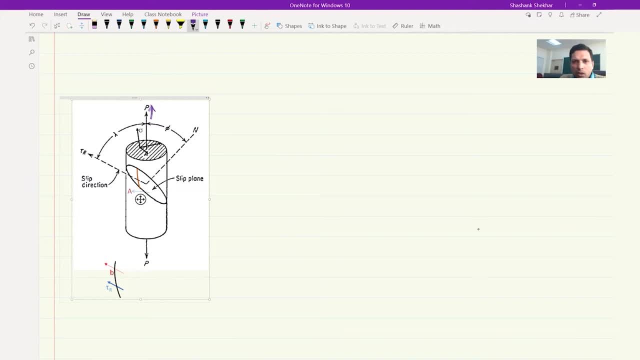 for the dislocation motion which, in turns, would mean the initiation of plastic deformation. So here we know that the angle between normal to slip plane, which is this normal to slip plane, is given by N and tensile axis. So this is the angle between normal to slip plane. 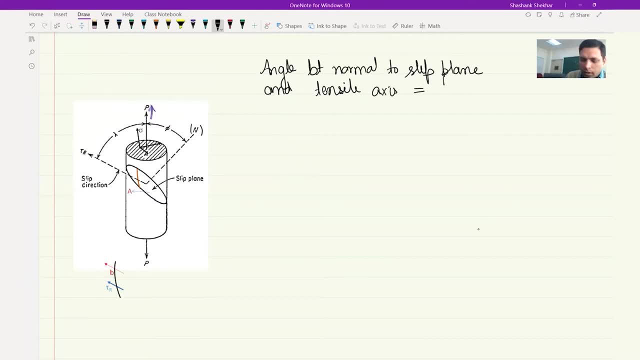 is given by N and tensile axis. So this is the tensile axis P and this is the normal. the angle between them is given by phi, So angle between the slip direction. So let us say this is the slip direction, meaning the Berger vector is like this: oriented slip. 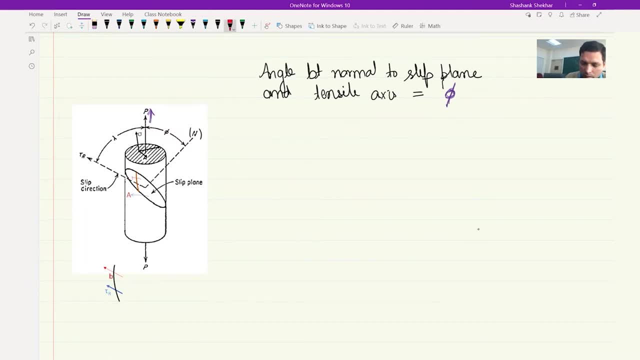 somewhere over here. So that will define the slip direction. So we want to know what is that angle between slip direction and tensile axis? And this is the tensile axis, This is the direction of the slip, or the Burgess vector, which is where the resolved shear stress. 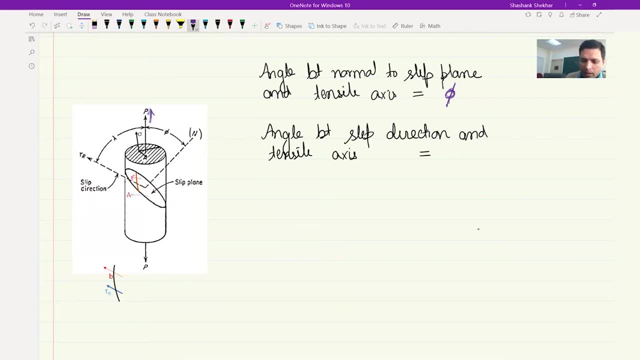 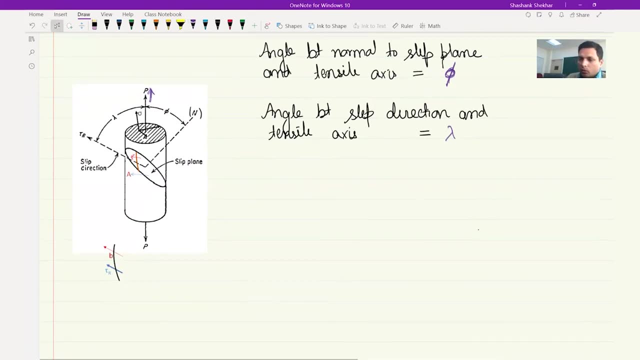 must act, And this is given by this angle lambda. now, if we know these two angles, we know a lot of information. let's see how. so now we have area of the slip plane. so if this is the system, then the area of the slip plane is now. so this is the slip plane. 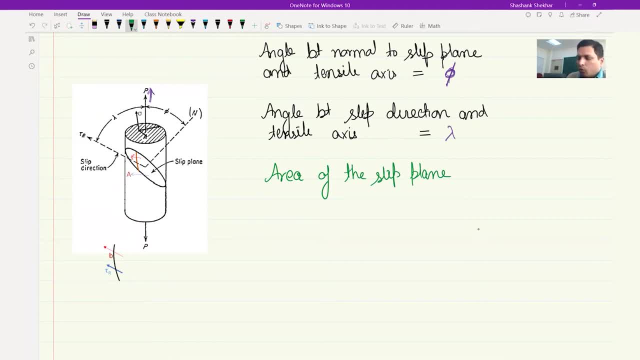 now, in this orientation, this oblique case, which would mean that the area of the slip plane which is inclined at angle phi is given by a, by cos phi, where we are, we, where we know that the original area, this, this area, is a, so this area was. 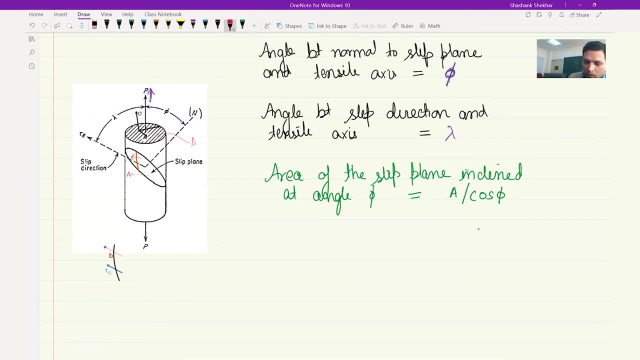 a, a, not this one, this is a by cos phi. the load, which is are the stress, p by a stress, was acting along this direction. so now we need to find the stress acting along the burgess vector, which is tau r. so that would be given by. 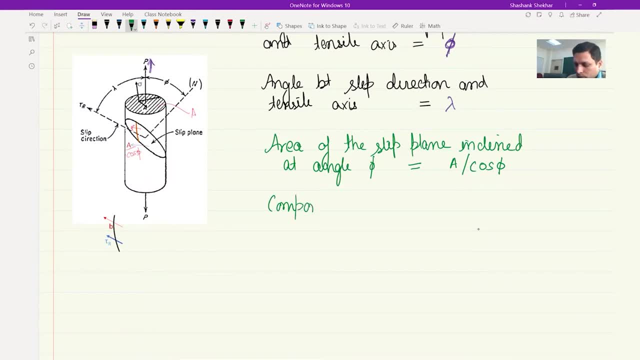 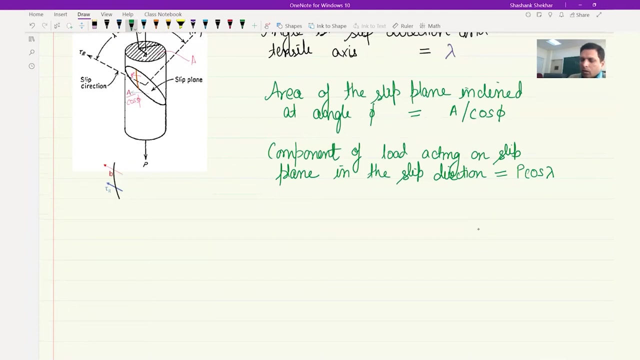 p by sorry t upon my sorry1, because it cannot be called t upon by for the tare. and so this says component of load. this would be: p is acting, and this disaster moment out here is acting in this direction. So cos lambda is equal to P cos lambda. So now we have the load. 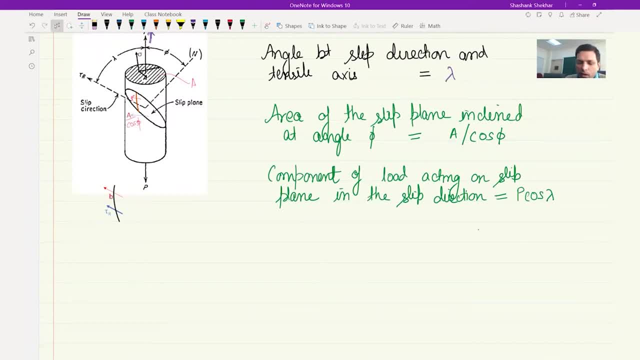 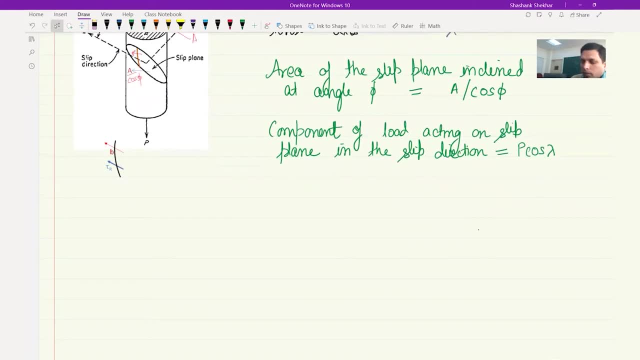 and we know the area and therefore we are in a position to find what is the stress acting here and therefore that would be given by resolved shear stress acting along slip direction on the slip plane on the given slip plane is equal to tau. r is equal to P cos lambda by A by cos phi, which is equal to T by A. 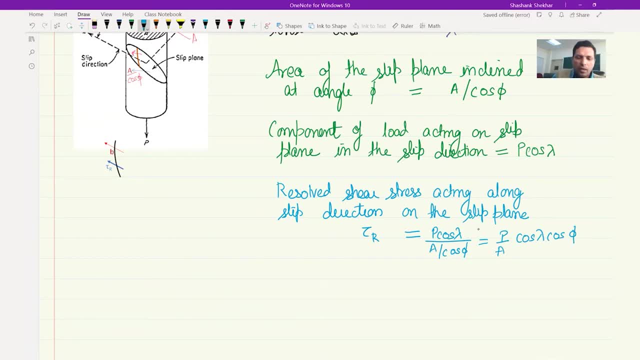 This is very similar to, or in fact it is along the same lines, where we are in a position to find what is the stress acting here. So now we have the load and we found, or where we did the axis transformation. Here also we are doing the axis transformation. 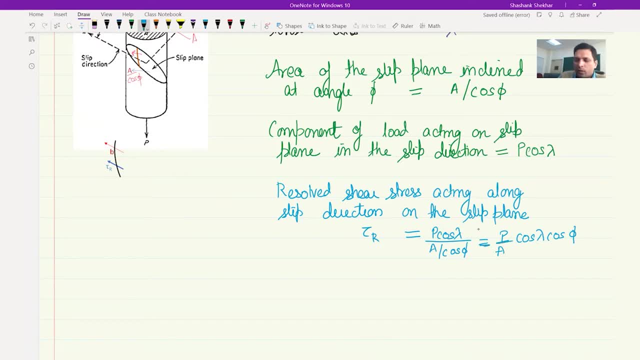 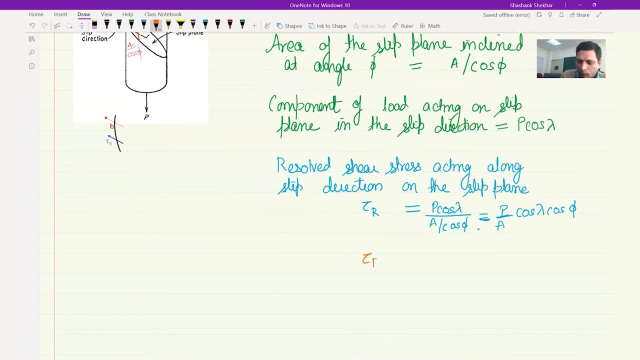 and of a particular quantity, and therefore you can see that the form of the equation is similar. Therefore, in the end, what we get is this: tau r is equal to P by A, we know, is sigma cos phi, cos lambda. So what this equation is. 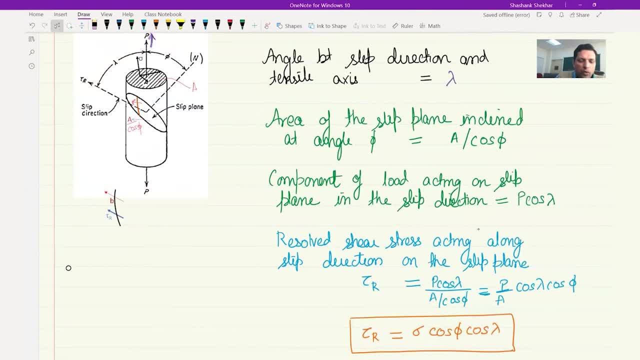 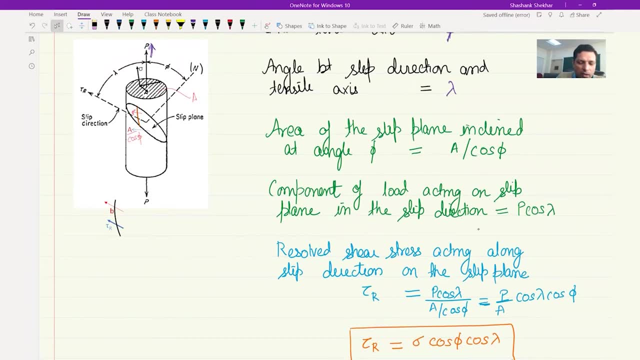 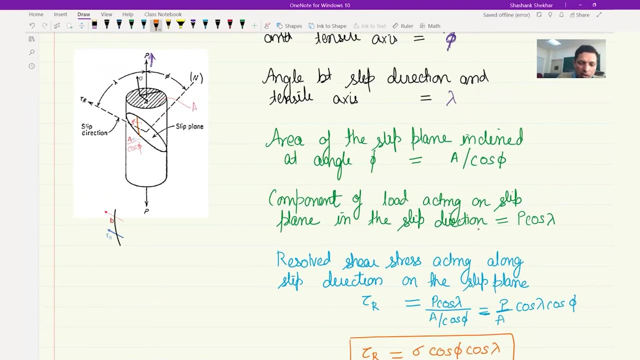 saying that if you want to find the dislocation stress or the shear stress acting on to this dislocation, where the Berger vector is along this direction and it is moving on this plane, where you are given that sigma or T by A is the stress acting along this direction, then 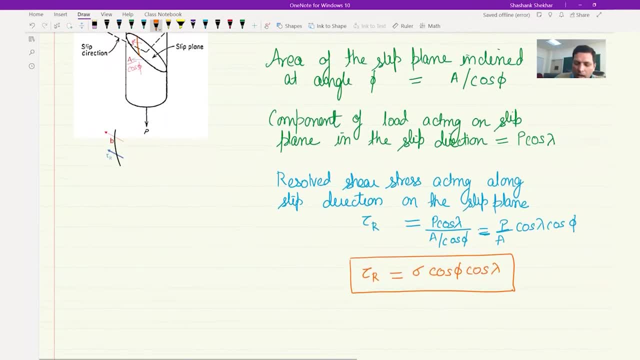 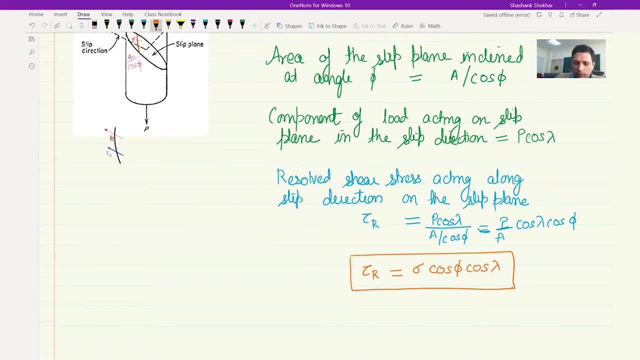 the shear stress on this particular dislocation would be sigma times cos phi, times cos lambda. That is what we obtained From this equation. So does this mean that once we have any amount of shear stress acting on the dislocation, the dislocation would start to move? The answer is no. You need a minimum shear stress along this. 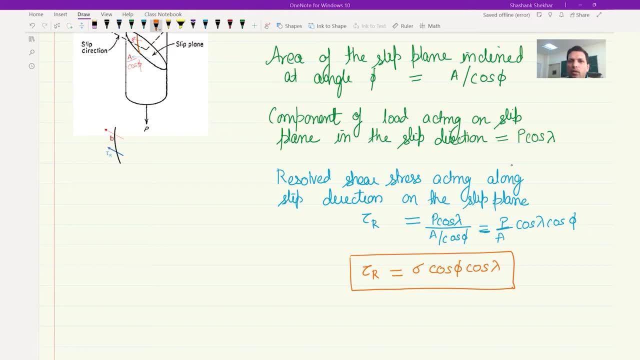 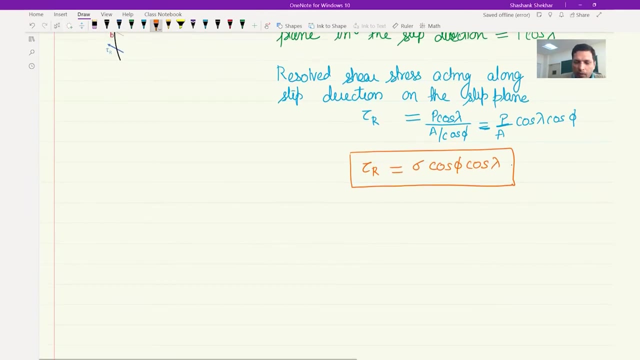 direction for the dislocation to move, which is what we call as critical result, shear stress, which we will get to in a moment. But before that, let us be very clear about a couple of things over here, and let me put it like this: So we have tau r. 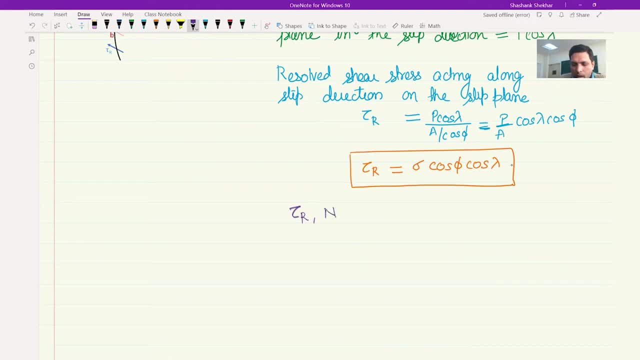 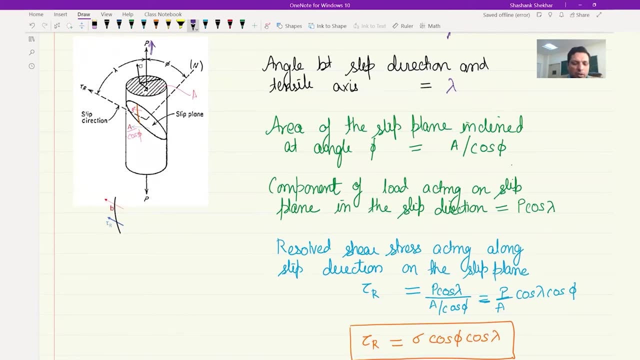 n, which is this one, and P. So we see in the image, in the two-dimensional image, it may seem like that tau r, P and n are all in the same direction. It need not. So this is something you have to be very clear about, that this tau r, P and n need not be in the same plane. 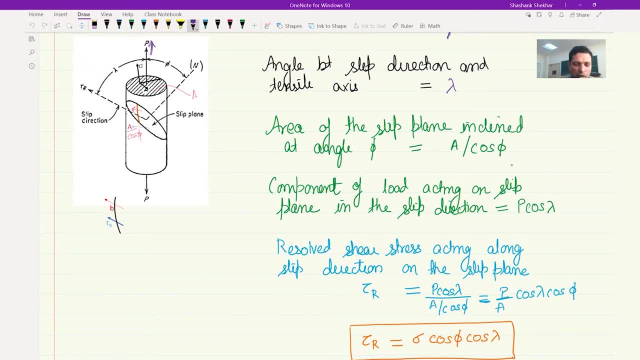 For example, the Basler vector could have been pointing in this direction. So this whole thing would have been rotated like this over here, and therefore tau r P- n would be here and the sorry, the P and n would be here, and the tau r and P would be like this: 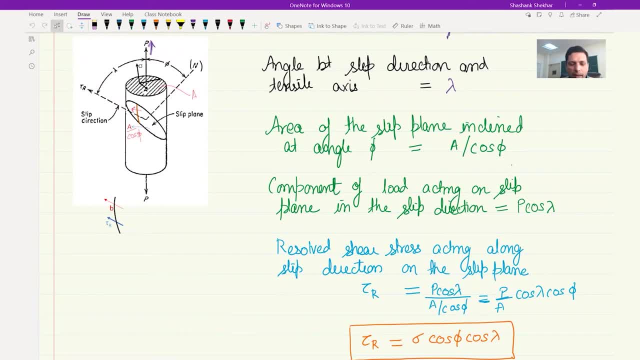 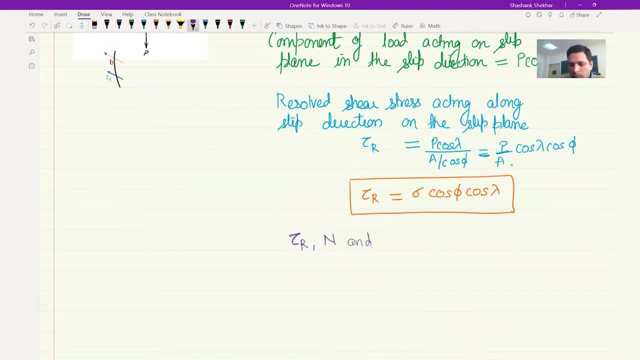 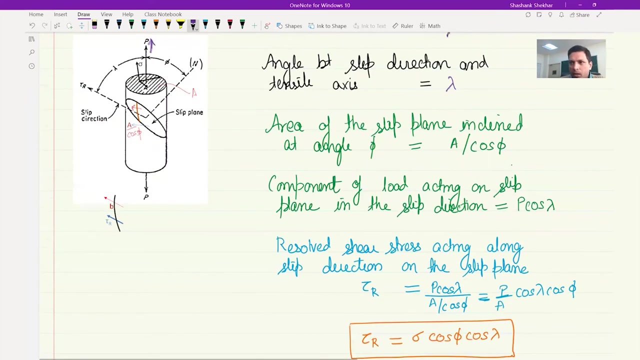 So in the general case, tau r P and n would not lie in the same plane, Need not lie on same plane, And the corollary for this is that phi plus lambda need not be equal to 90 degree. In fact, that would be a very special case where phi plus. 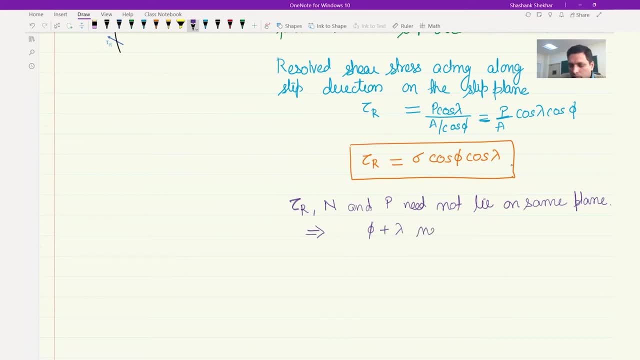 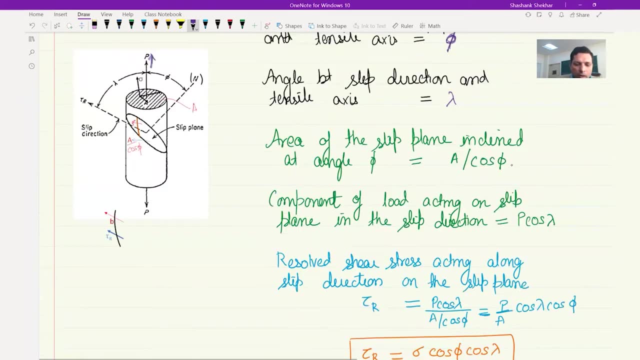 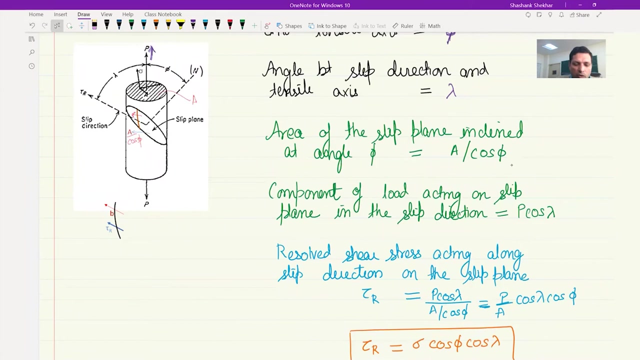 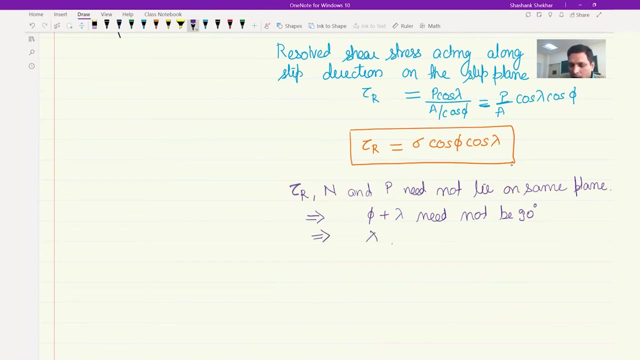 lambda is equal to 90 degree. Even lambda, in some orientation of this drawing it may look like lambda is equal to 90 degree. So let us be very clear about that too, that no, lambda need not be 90 degree. Of course, in some particular case it can be 90 degrees. 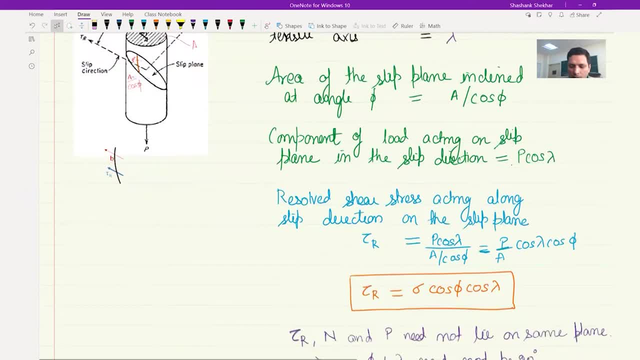 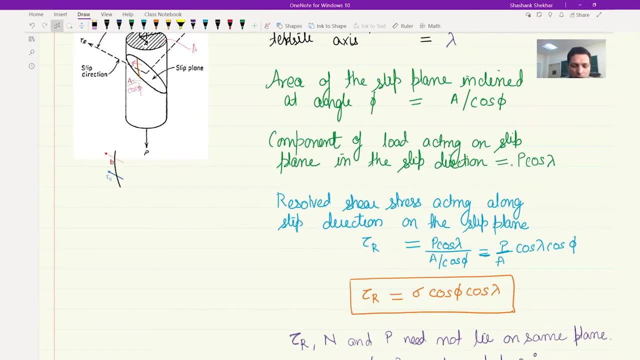 So with this we have now resolved or found a relation to find what would be the resolved shear stress acting on a dislocation with a given Berger vector which is oriented where the slip vector or the Berger vector is along this given direction. So we all 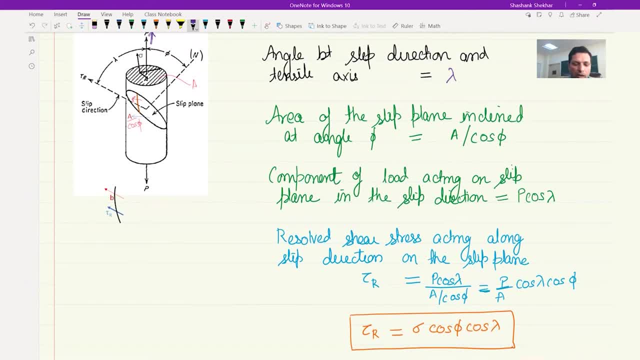 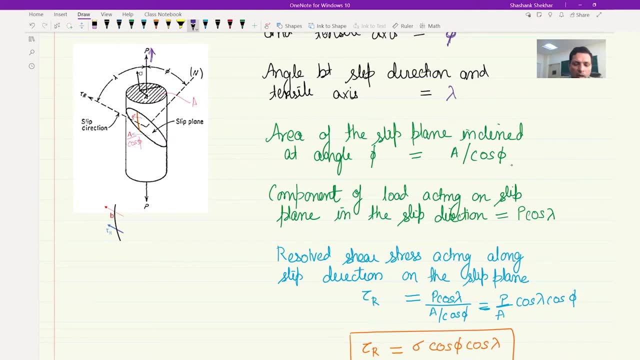 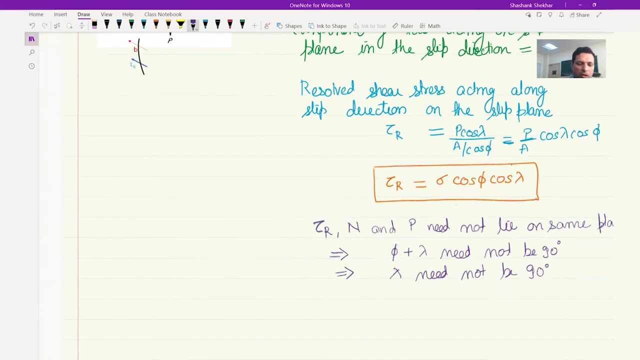 we know all these vector with respect to or in terms of the angle. So the Berger vector is oriented with respect to P at an angle lambda and the plane normal is oriented with respect to P at an angle phi And, like you said, this is tower. but just because the 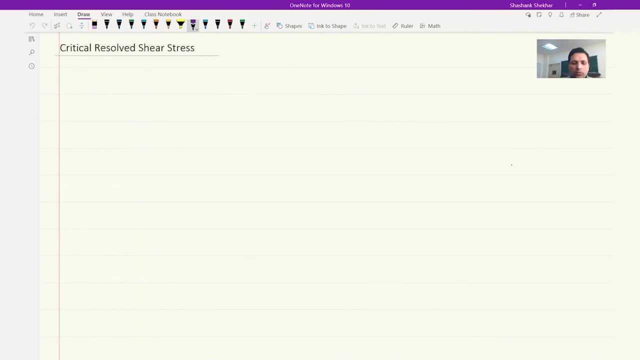 shear stress is being applied, it does not mean that the dislocation would start to move. We need some critical value for the dislocation to move. 4- So what is that critical resolved shear stress. So this is the minimum, The minimum value of tau R. so tau, this will be called tau CRSS. The minimum value of tau R. 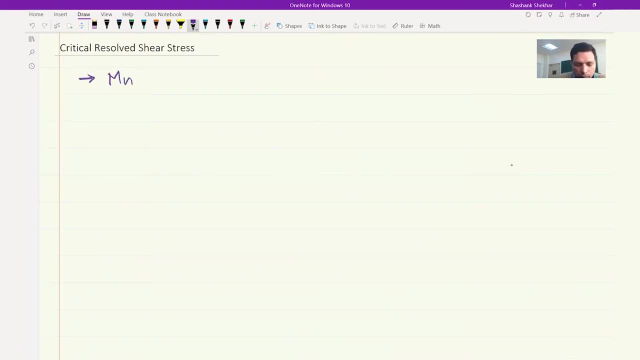 will be called tau CRSS. So the minimum value of tau R will be r to 3 times tanks c to the front right. in the slide, Just in JA, And I am using that r means the minimum value of t of tau C to the front right. so t I will like to keep Sen I have used here 10. 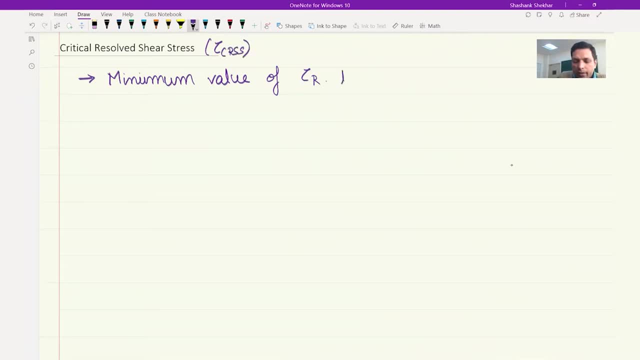 until now. otherwise I am interested in the last Limit. The value of this s and that c will be called one to the right minus number d to the left. to the left, The minimum value of tau R and t is applied tau c to the, the height. So it will be this здесь This is called theultra. 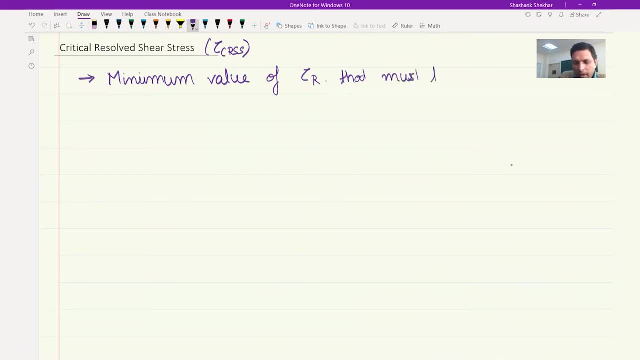 that must be applied for dislocation to move. so this is minimum value or a threshold value and the critical result- shear stress- is a minimum or critical or theoretical threshold that tower must reach before the dislocations can start to move, and what it implies is that if tower is less than this critical value, 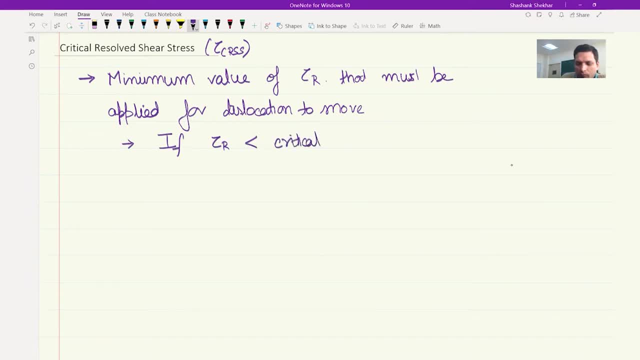 and then there is shear stress on the plane, but it is not enough. and also there is force on the dislocation, but it but dislocation does not move. so tower must be equal to or greater than this critical value before the dislocation starts to move. tower, what now? what is tower? it is a variable which is dependent upon applied stress geometry. 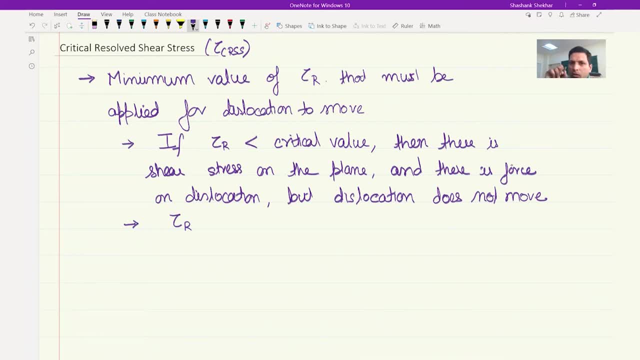 of the crystal and orientation of the slip. and so we saw it is dependent on sigma, it is dependent on cos phi and cos lambda. on the other hand, tau crss the critical result, shear stress. it would be a fundamental property of the material, just like the yield strength. 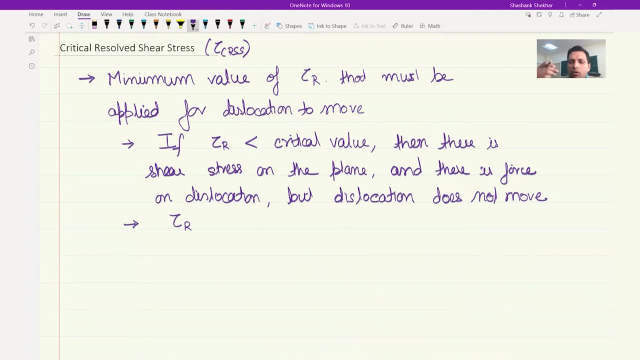 so yield strength is something we describe it with respect to polycrystalline materials. but in single crystalline material and for a given slip plane we will define it in terms of tau crss or tau critical result, shear stress. so tower is a variable, so it keeps changing, not tau crss. tau crss is one quantity. 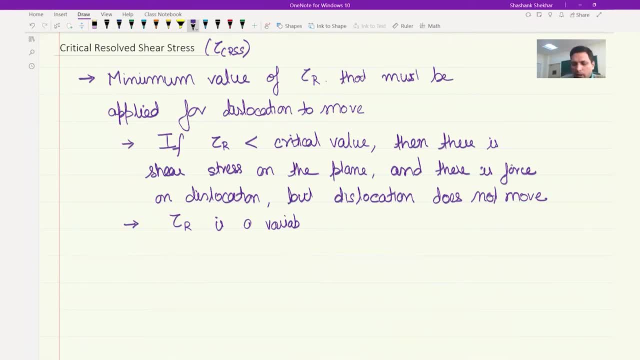 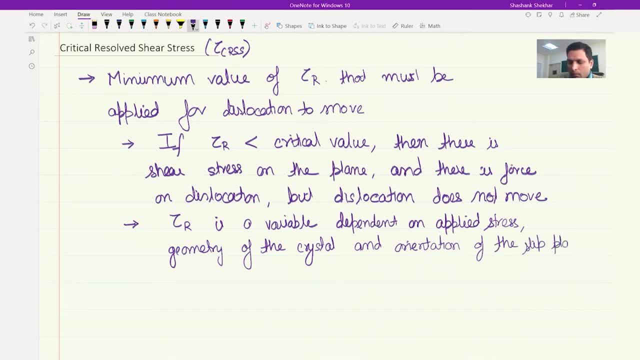 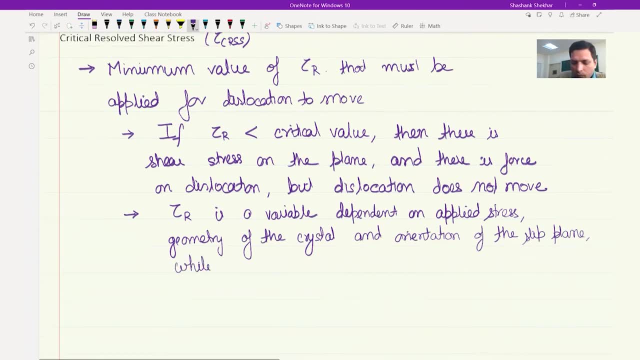 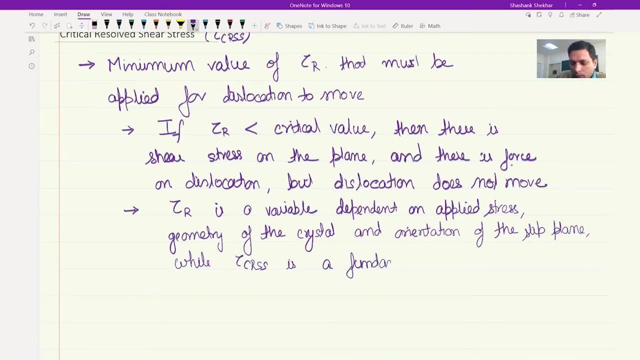 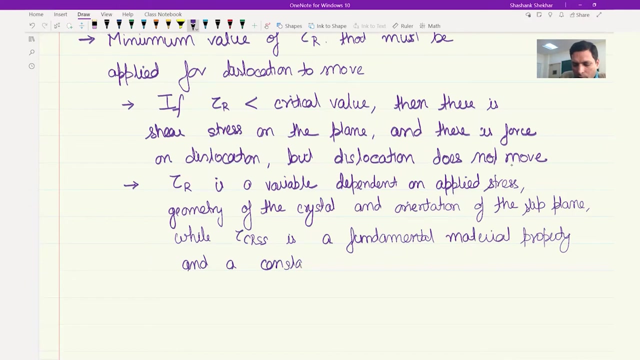 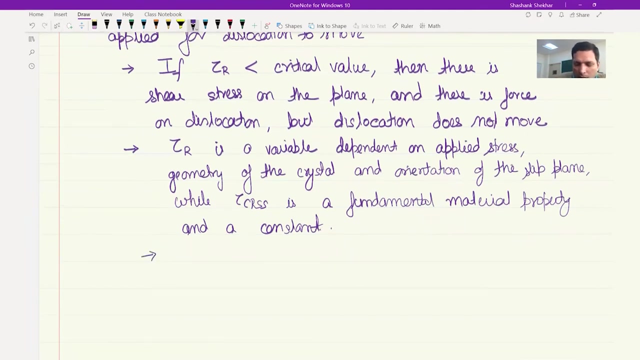 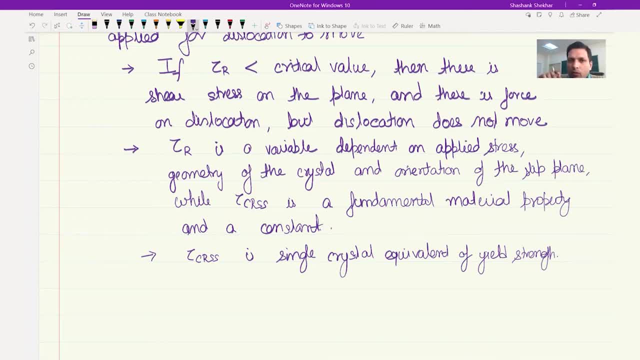 reaches this tower, reaches a critical value, which is what we call now as tau CRSS, then dislocations start to move and yielding takes place. So the overall relation for tau CRSS would still be defined like this: tau CRSS is equal. 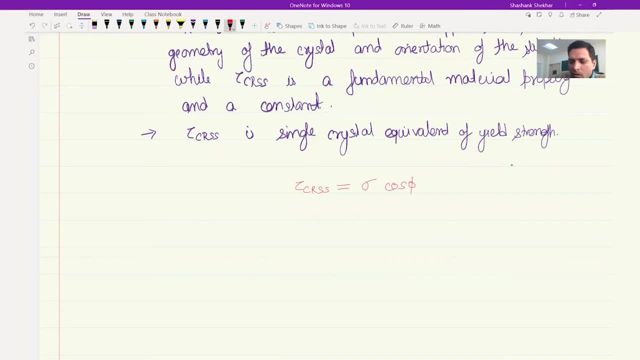 to sigma cos, phi, cos, lambda, but then this would be a particular value, and this is one particular value where the dislocations start to move. So it is for the given phi and lambda, whatever the sigma comes out to be, that would be the. 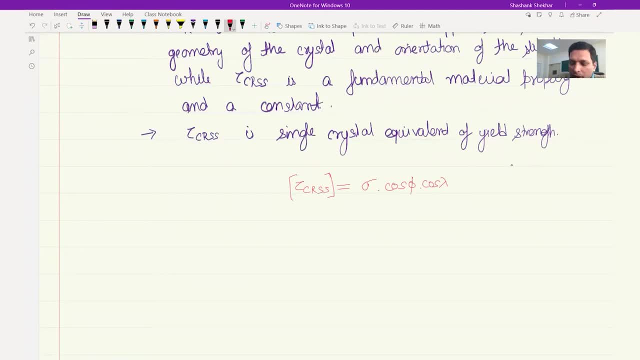 stress at which the dislocations start to move And, in fact, this sigma would be determined using this value: tau, CRSS And for all other values, what we will say That tau R, whatever value we get from this relation, is equal to the resolved shear stress. 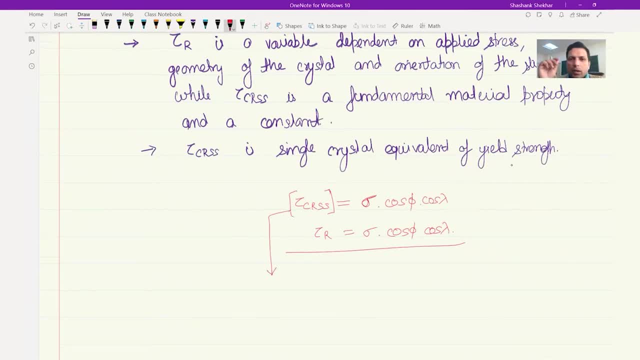 So tau CRSS, as you have seen, is a critical value where the dislocations start to move. But then it will probably also remind you of another parameter that we had studied a little bit earlier. that was called the Payjean-Baro stress tau pn. 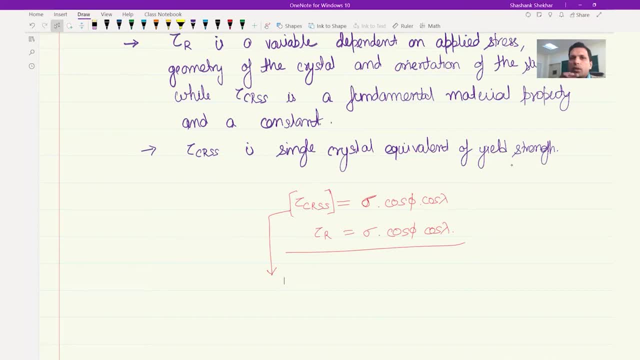 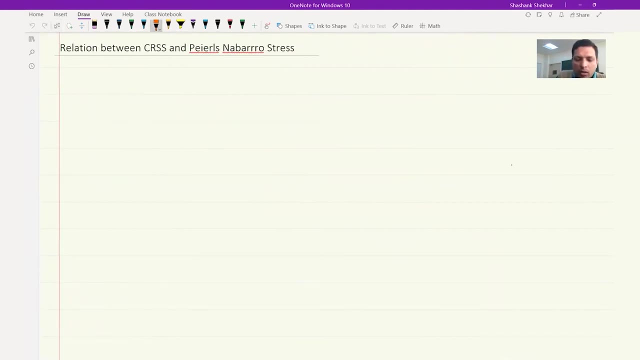 And that was also the stress at which the dislocations start to move. The question is: what is the relation between this CRSS, the tau CRSS and the tau pn? So we want to understand what is the relation between tau CRSS and tau pn. 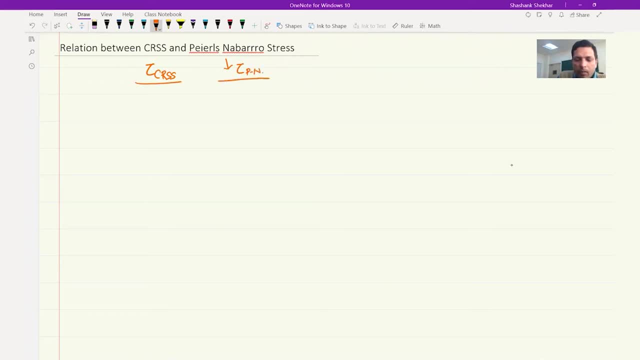 Any other questions? n. so what do you think? are they the same thing, are they something completely different? or they have no relation amongst each other? so it so happens that both these quantities reflect the minimum shear stress. why we are actually discussing it here is for this reason that both these quantities 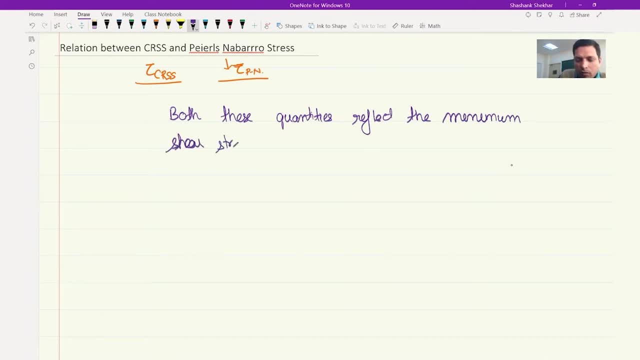 minimum shear stress to overcome less shear stress. to overcome less shear stress, to overcome lattice resistance. in taupean also. we saw that there is. there are these per in taupean also. we saw that there is. there are these per in taupean also. we saw that there is. there are these per energy valleys. 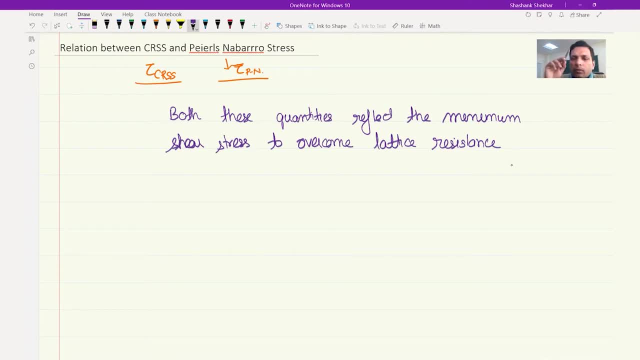 energy valleys, energy valleys, and we derive from that, or we can derive from. we derive from that, or we can derive from. we derive from that, or we can derive from that energy values, that energy values, that energy values. by that, by taking the first differential, by that, by taking the first differential. 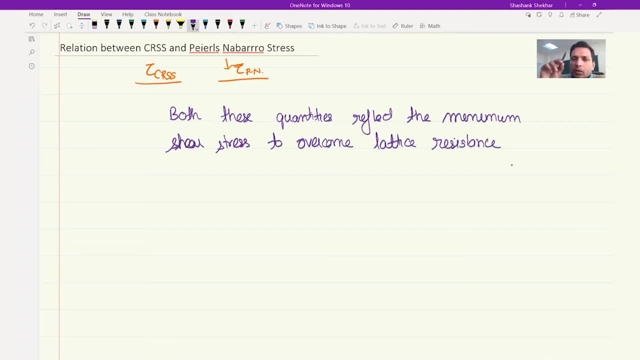 by that, by taking the first differential, we can find the shear stresses. we can find the shear stresses. we can find the shear stresses and and and those shear stress. if you took look at those shear stress, if you took look at those shear stress, if you took look at the amplitude. 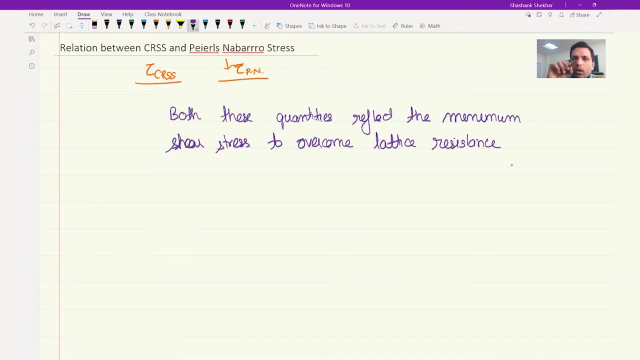 the amplitude. if your shear stress, overall shear stress, is less than the amplitude, then it would mean that you will not be able to come out of the value and therefore the minimum shear stress that you need to apply is the equal to the amplitude, and we that is what we called as tau p? n. so that is also the 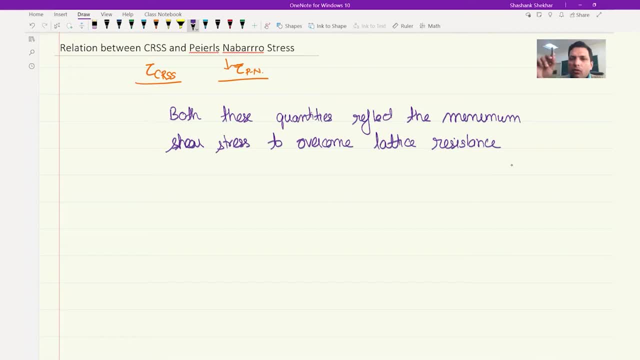 minimum lattice: uh, the minimum shear stress that you need for the dislocation to move against the lattice resistance- and here also we look at the tau? p? n- is the shear result, shear stress along the dislocation, but it will not move unless it is over and above some critical value, which is what 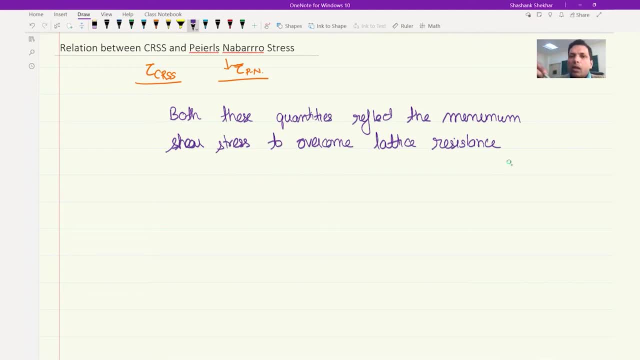 we call as tau crss. so below this, it is as good as saying that it is inside the valley. and when you apply stress higher than this critical value, then the dislocations start to move. so what is the relation? that is the question, and the answer is that actually both of them are. 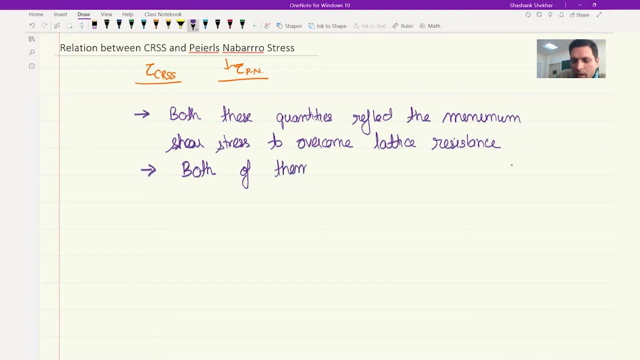 both of them represent the same phenomena, the same i wouldn't say phenomena, but both of them represent the same quantity. however, there is a slight difference between the two and it is given here. so tau p n is actually a theoretical quantity. we can use it and this is the theoretical quantity we are talking about in the theoretical model. 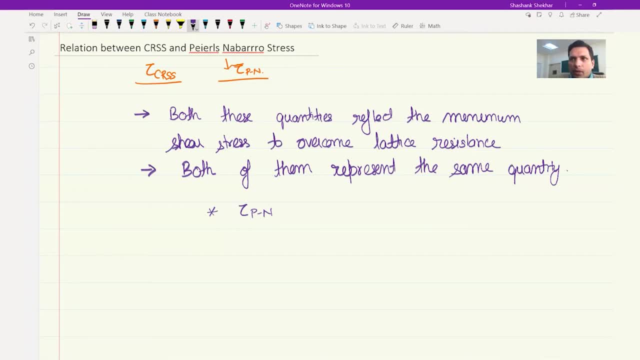 so you see, we obtain that based on theoretical model, and in that theoretical model we have not taken into- at least until now, we have not taken into account temperature. so tau p n is a theoretical energy or, sorry, theoretical stress that is required for dislocation to move, and also that it 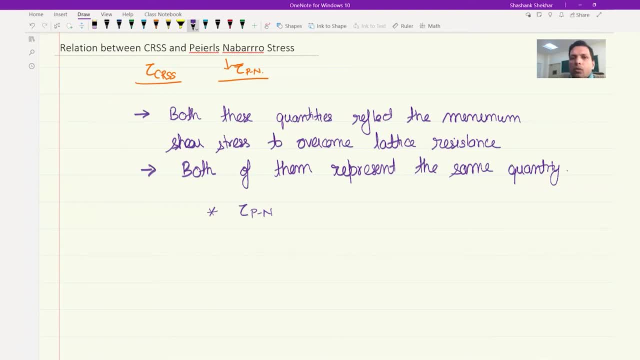 the equations that we have dealt with. On the other hand, tau CRSS is an experimental quantity and therefore, whatever temperature you are doing the temp test, it represents the resistance at that particular temperature and therefore it is a temperature dependent quantity. If you do it at 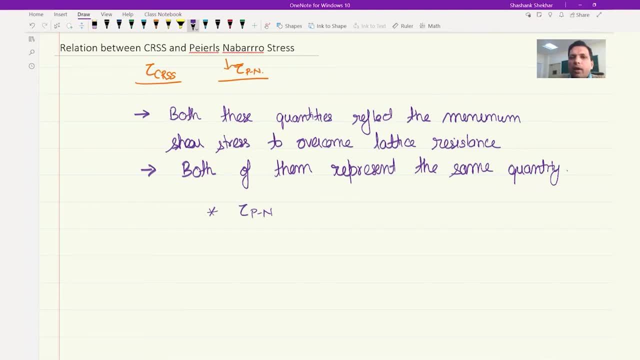 very low temperature versus at very high temperature, you would get different values of tau CRSS. So that is the main difference between the two. However, both of them represent the same thing, that is, the lattice resistance of the lattice resistance against the movement of the dislocation. So let me summarize what I just mentioned. Tau Pn is a 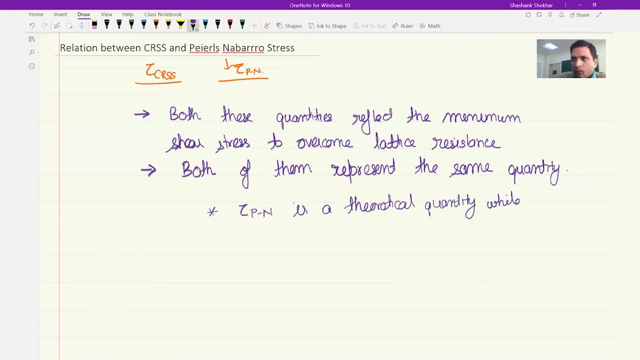 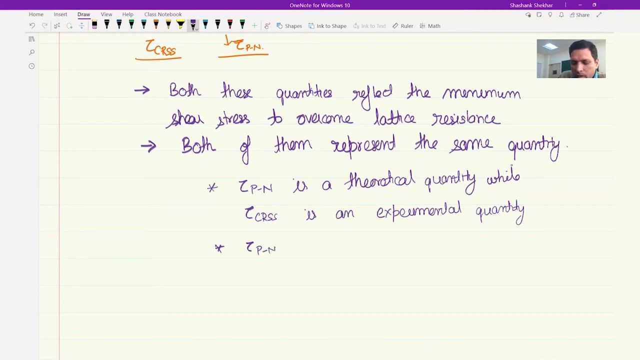 theoretical quantity quantity, while tau CRSS is an experimental quantity. Tau Pn is given for 0 Kelvin, while tau CRSS is obtained for a given, whatever temperature you have done. So that was the second difference. Another proven differential point is all the specific values of tau CRSS. 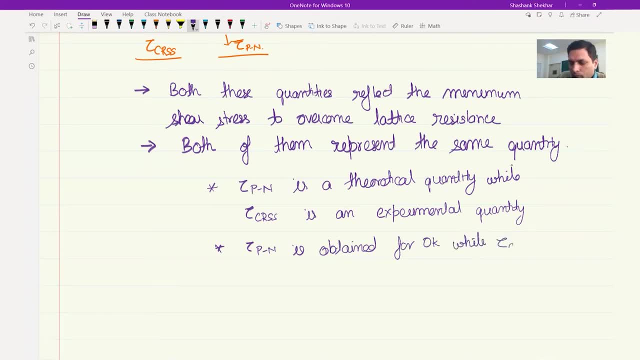 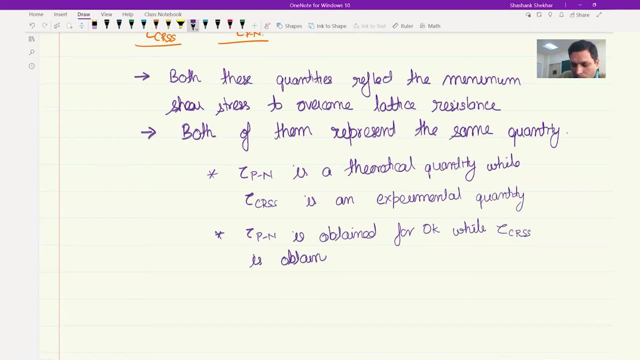 that is, if the temperature is at low temperature versus high temperature, then Phoenix temperature increase. what do you mean? or what? what we assume that the temperature is? So this is the relationship PMU test that I already showed in previous video. We were actually having an intranet plate clock called. 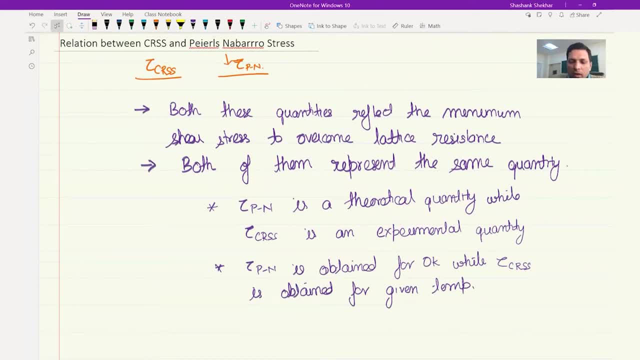 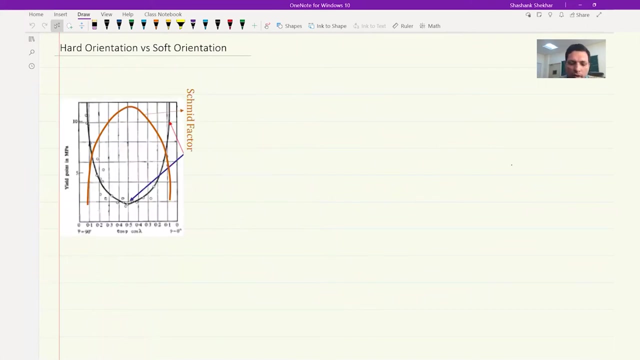 So this is the relation and we must keep this in mind because it is not that we are talking about two different things. So, with this understanding, now let us move on to understand another aspect about this: resolved shear stress. And we have looked that there is a factor: cos phi into cos lambda. 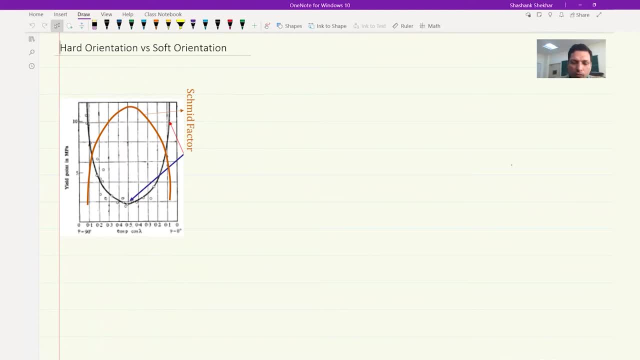 Now this factor, cos phi by cos lambda. this can be termed as m or equal to. so cos phi into cos lambda, which is also called as smid factor. Now, if you look at the relation again that we had obtained, So tau r is equal to: 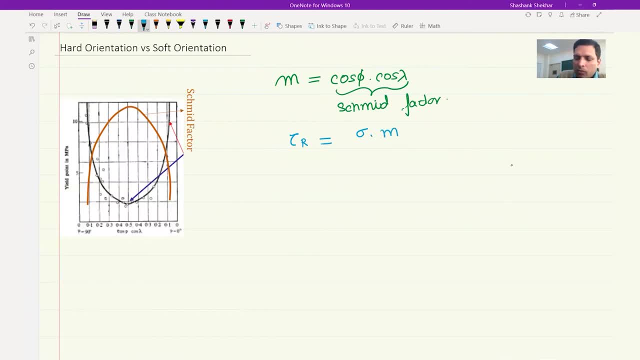 So tau r is equal to sigma times cos phi, cos lambda or m, And if it happens to be CRSS, then sigma is given by tau, CRSS by m, Meaning that this stress that you need to apply for the dislocation to move on a given plane would be lowest when m is highest. 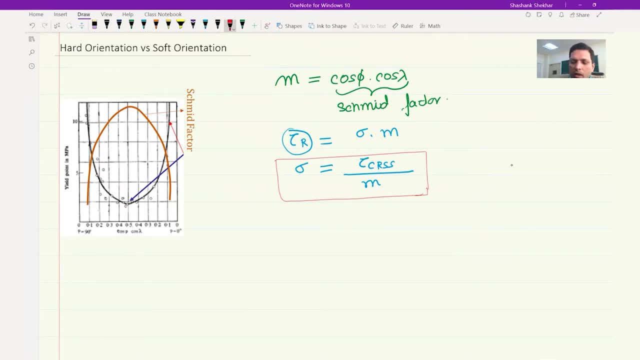 And when is m highest? When cos phi comes times, cos lambda is highest. So people have done experiments where they have changed the values of phi and lambda. So you get here this is done, where phi has been changed from 0 to 90 degrees and cos lambda was kept constant, so that your cos phi to cos lambda values changes continuously. 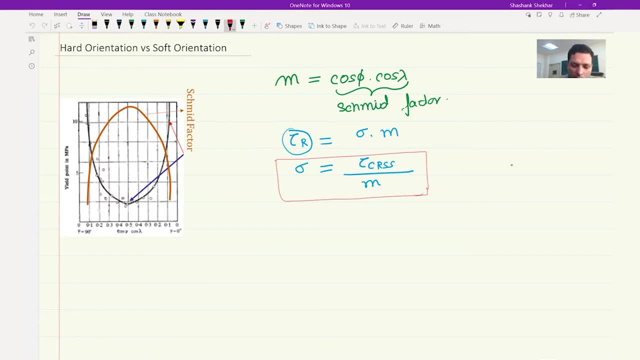 And what you can see is that when the cos, phi, cos lambda value is, the angle is somewhere close to 45 degrees, that is when you would get the lowest value of the yield strength, and if you were to draw the mid-factor values, then it would actually be. 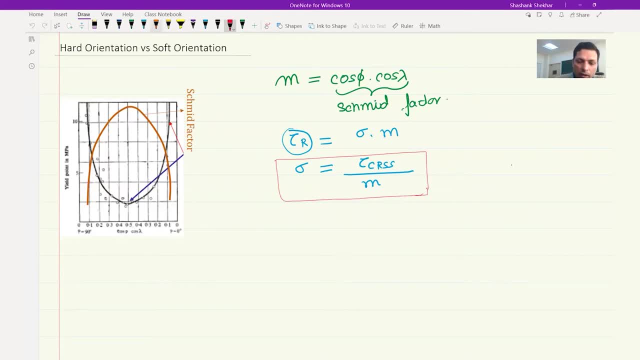 the inverse of this. so this will be highest over here. so this is the highest value for m and at the same point you would get lowest value for sigma. so the planes which are oriented close to 45 degrees would give you the or. there you would need the lowest. 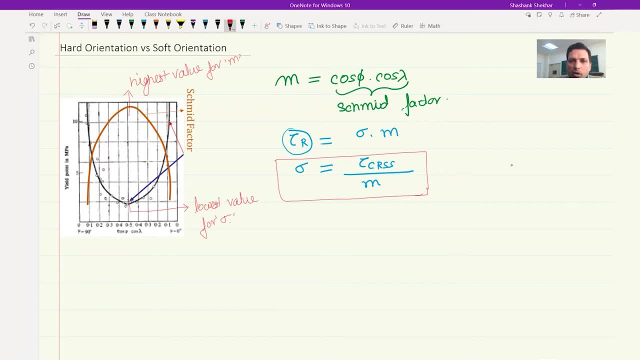 stress, the tensile stress for the dislocation to move. and this is in line with what we have already observed, that when you apply the tensile stress, then along the 45 degree planes you get the highest shear stress. so this is, you can say, corollary of that, because the shear stress is 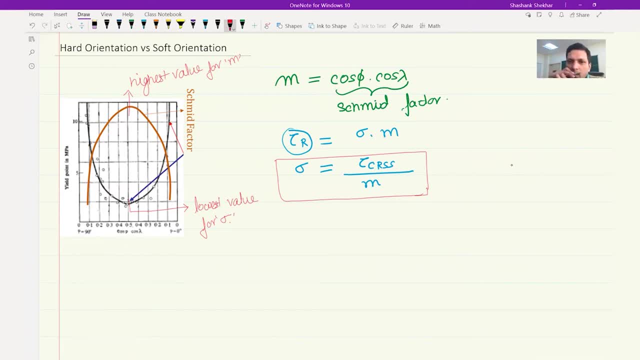 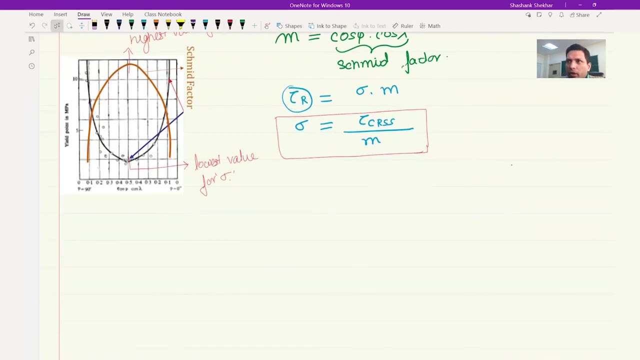 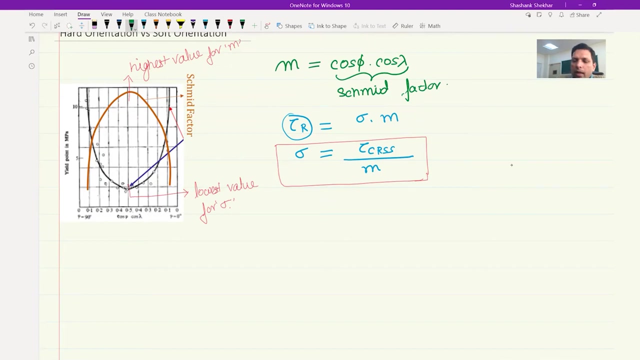 highest over there. that is where. that is why the planes oriented close to those 45 degree planes would show the lowest value of yield strength. and a corollary of this we can look at this is over here is like this: so when can we get the highest value of the cos phi, cos lambda? when the angles are lowest. so for maximizing. 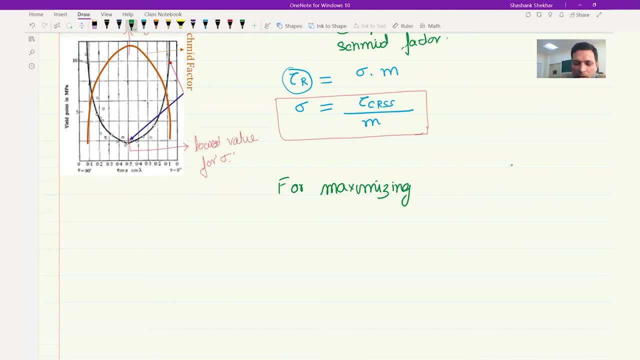 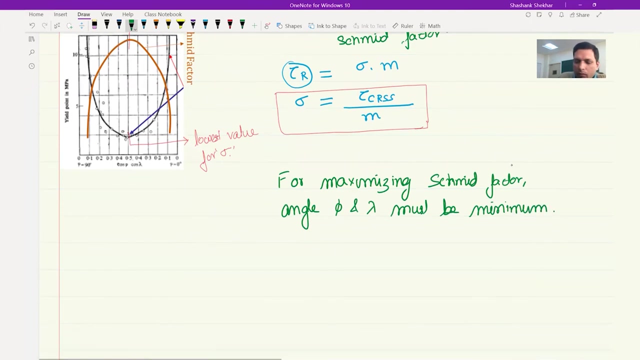 so we will show quantitatively that this is this. lowest value of yield strength and highest value of smith factor would actually be obtained for 45 degree. so for maximizing smith factor, angles, phi and lambda must be minimum, and it is minimum. so far we have assumed that they can be in different planes, so phi can be. 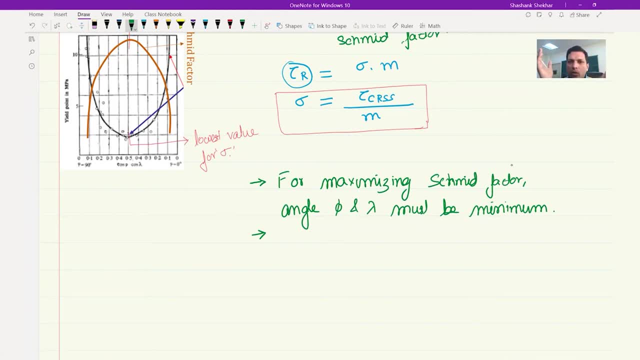 in one plane and then they can be in another plane, and then they can be in another plane and lambda can be another plane. but if you want the total to be minimum, then these two must become together or it must be in same plane. therefore, it will be minimum when all 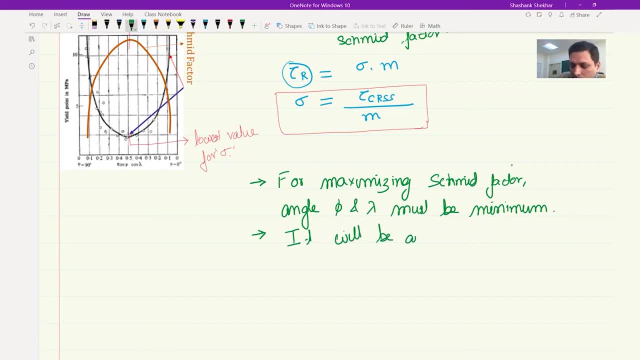 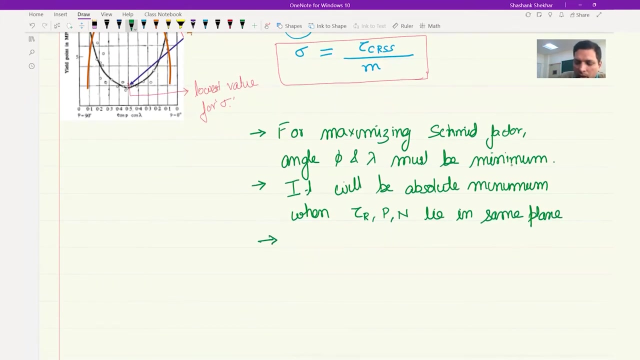 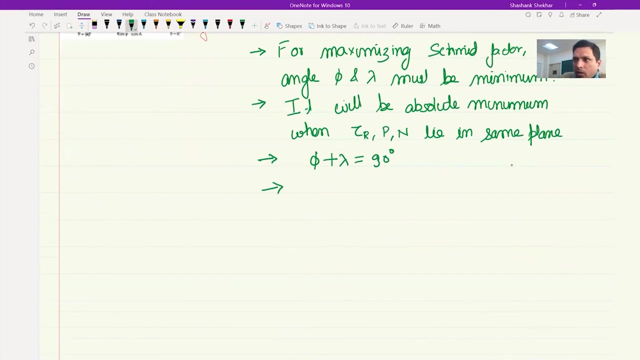 it will be absolute minimum only when, when tau r, p and lie in same plane, and when that is the case, that would mean that phi plus lambda is equal to 90 degrees and hence maximizing cos phi, cos lambda. you can now apply the simple mathematical rules to maximize the cos phi times cos lambda. 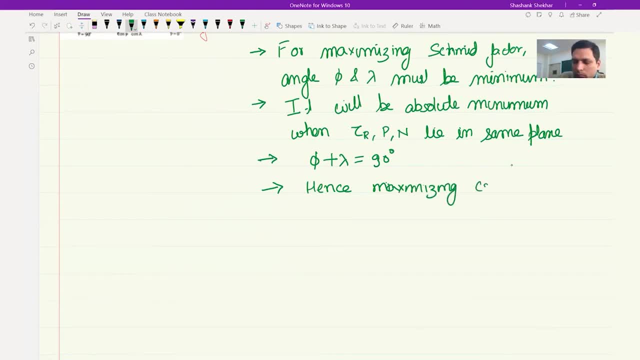 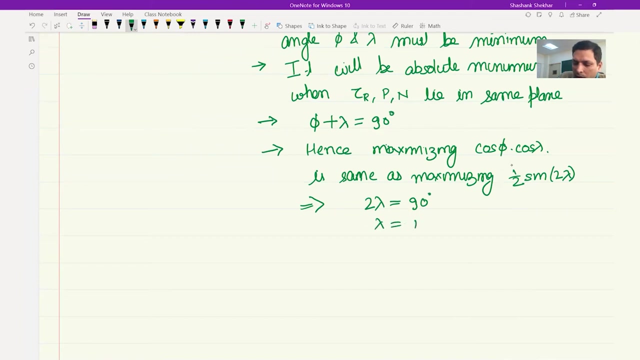 is same as maximizing 1 by 2 sine 2 lambda, because now they are related by this relation and it implies that 2 lambda is equal to 90 degrees. or lambda is equal to 45 implies phi is also equal to 45 degrees. so you see, we have. 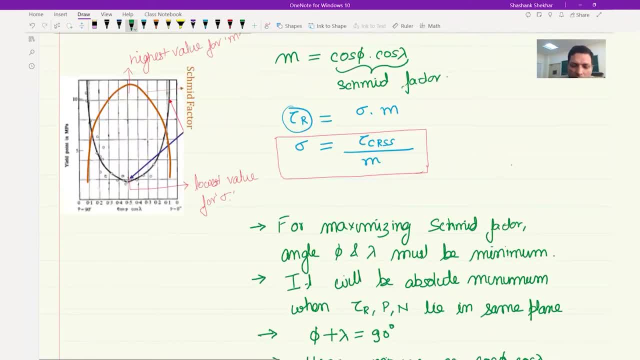 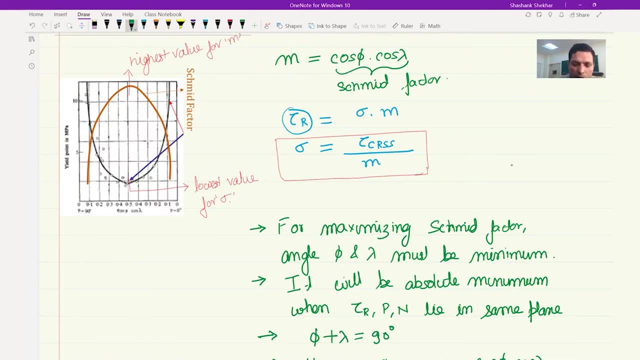 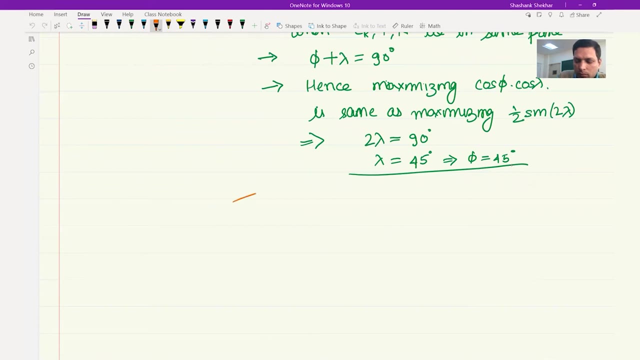 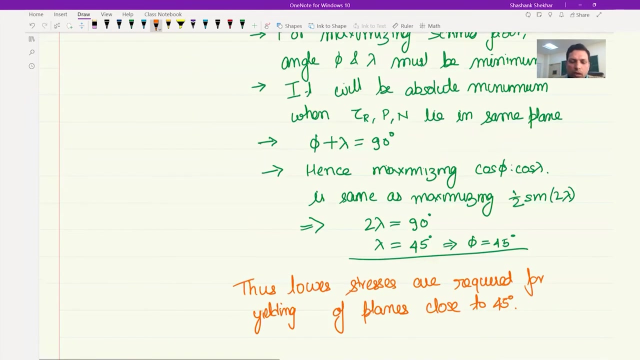 mathematically obtained, that smith factor would be highest when phi is equal to lambda, is equal to 45 degrees and at that time, at that particular configuration, you will have the lowest yield strength values. thus lowest stresses are required for yielding of planes close to 45 degrees. now here we have taken configurations such that some planes were 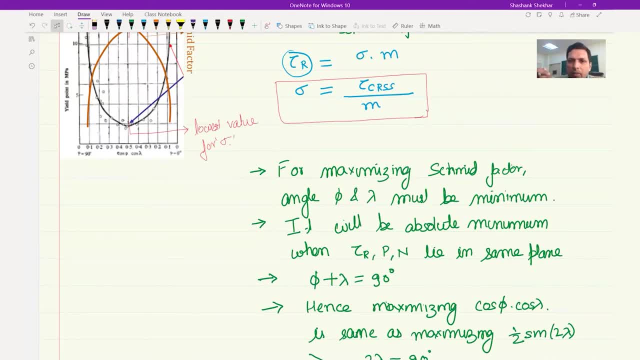 coming at 45 degrees. however, in practice, depending on what orientation of the crystal you take, not, it need not be necessary that some planes are actually oriented close to 45 degrees, which means there is no slip plane at 45 degree orientation. so what it means is that all the planes closer to the 45 degrees would be the ones that would this this. 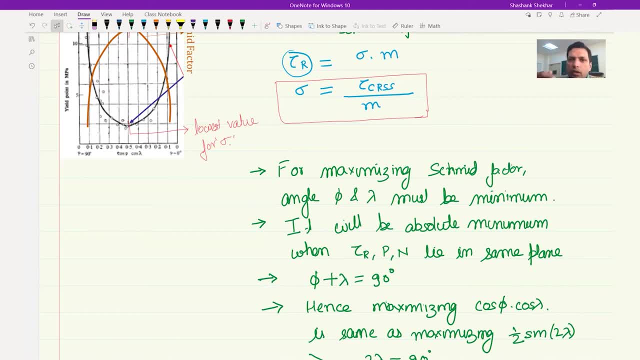 is what this drawing is showing- will lead to the lowest yield strength, or with this. these are the planes where plastic deformation or dislocation motion would begin, if at all. there is a possibility that there is a slip plane at 45 degrees, then of course the dislocation motion would take place. 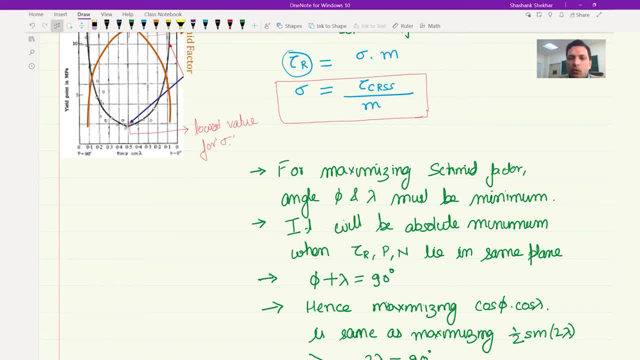 over there. but if not, then the ones closest to 45 degrees would be the ones where dislocation motion would take place. and, as i mentioned earlier, just a few minutes back, that this is also a corollary of what we had seen earlier, that when you apply normal stresses, the maximum shear. 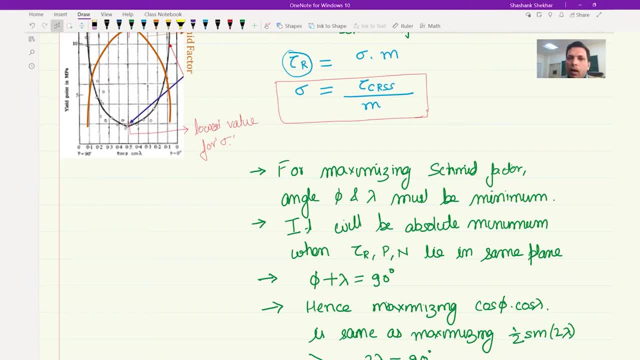 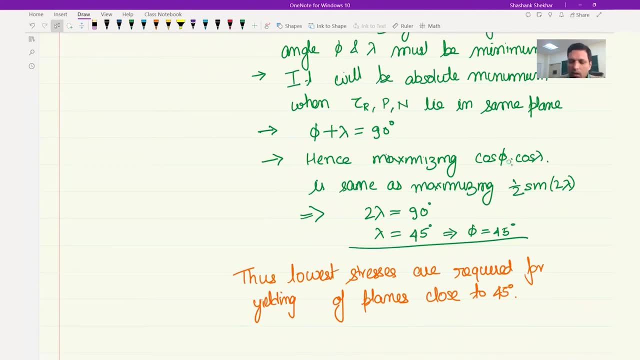 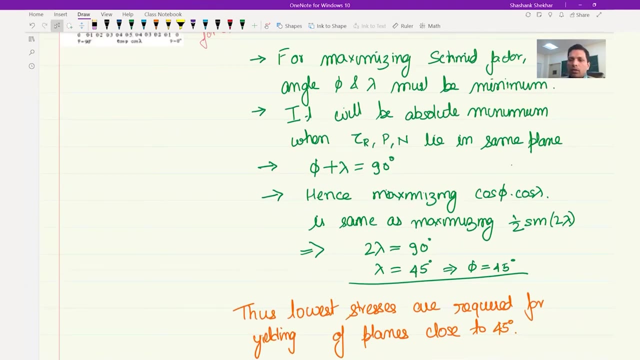 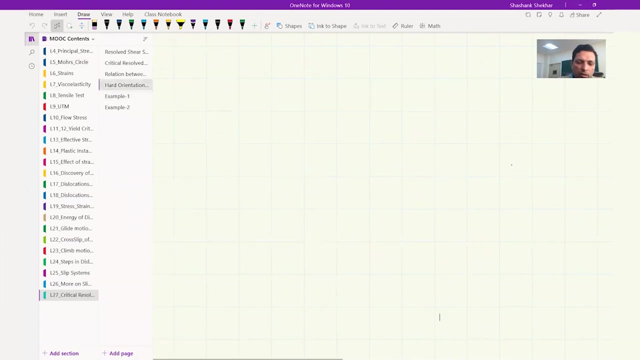 stress is at 45 degrees, so this is a artifact of this. so now that we understand this, now let's okay. okay, i've missed t here, so now we are in a position to look at certain examples, so let's try to solve some problems related to this, okay, yeah, so one point, i missed that i wanted to say which. 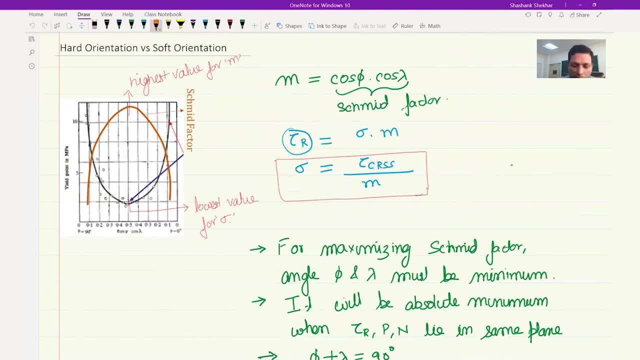 is the topic here: hard orientation versus soft orientation. so the orientations which are close to the this region would be called the soft orientation, meaning you need less stress for the dislocation to move along those planes, while the orientation which would be over here would be called hard orientation and in fact at zero degree or 90 degree, those would be called very, very hard. 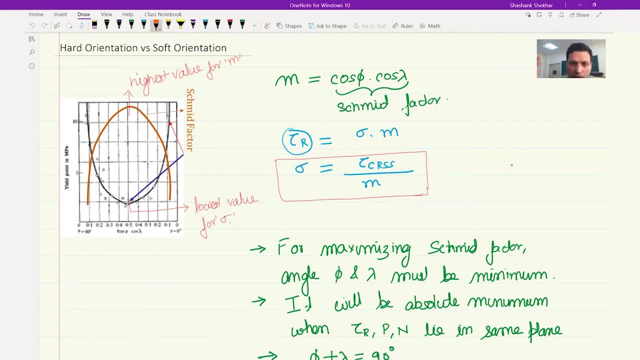 because you cannot. no amount of stress, the tensile stress, can make dislocations move on a plane, which is just normal point, because the simple reason is that there is no component of load which would be stress which can lie on this particular normal plane. because there is no component, and so you need the stress to move along those planes. 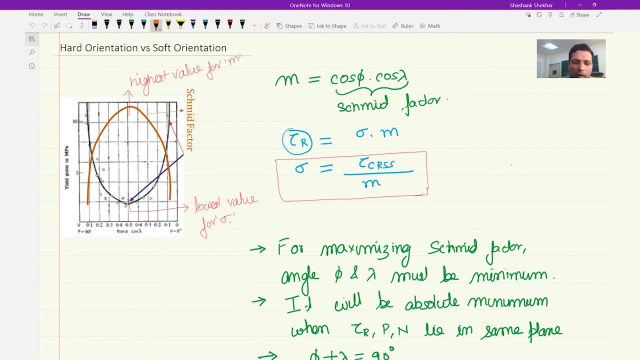 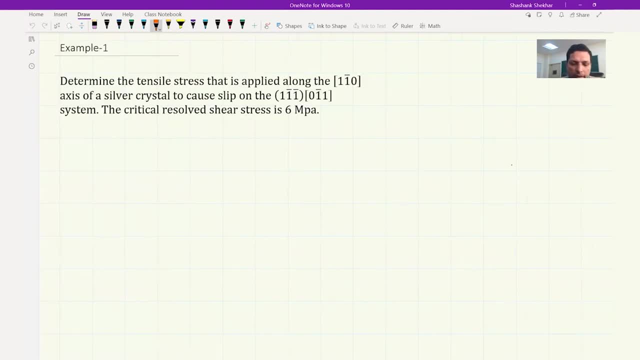 which would be called hard orientation, making a tendency order which hadn't reached the point where normal to it. so that is the reason that makes it hard orientation. okay, so with that, now let's try and solve an example. so the question is: determine the tensile stress that is applied along the 1? 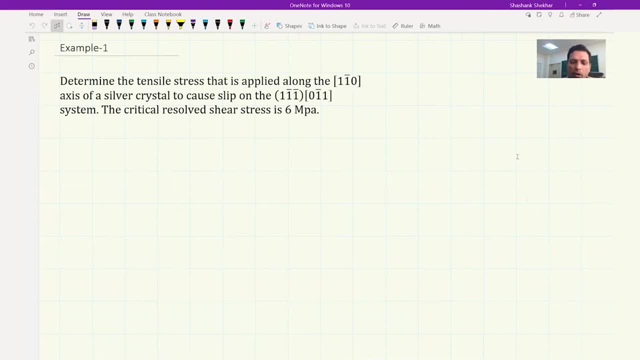 bar 1: 0 axis of a silver crystal to cause slip on 1 bar, 1 bar. 1 0 bar 1: 1 system. so basically, this is telling you the plane on which the dislocation is and this is telling you the slip vector it is. 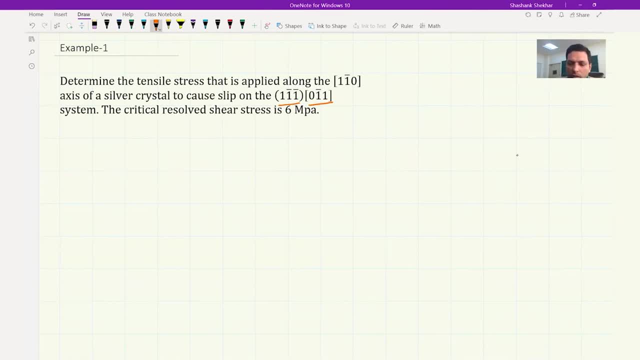 not the Burgess vector, just the slip direction. so Burgess vector would be probably a by 2, 0, 1, 1, 0 bar 1, and it is silver. so we already know it is the FCC system and the stress is being applied along 1 bar 1, 0. so just for the sake of completeness, let me 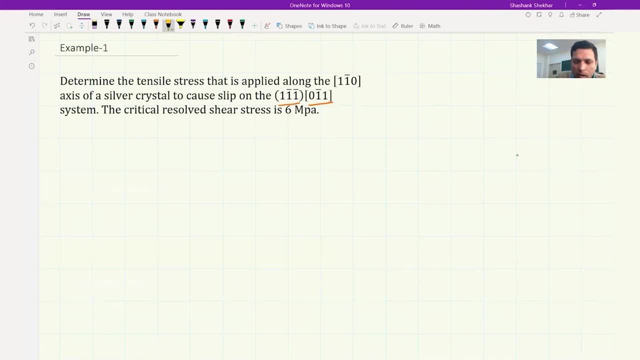 let me draw the overall configuration. it would look something like this: so this direction is 1 bar 1: 0, and there is a plane which is 1 bar 1, 1, and let's say there is a dislocation over here and let's say the Burgess vector is like this: so this direction would happen to be 0. 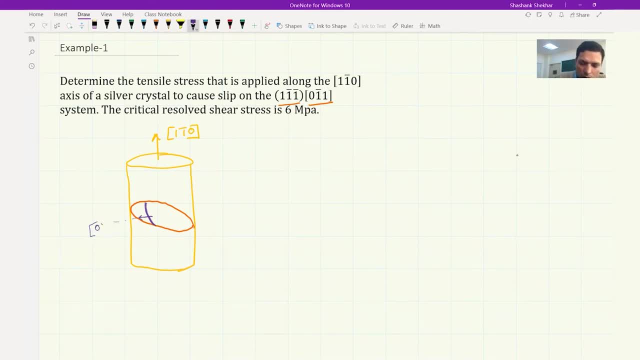 1 bar 1. so that is the overall configuration that you have been given. this is the normal, which would be 1 bar 1 bar 1, and we have said that this is the. so let's say: this is the phi and this is the lambda. 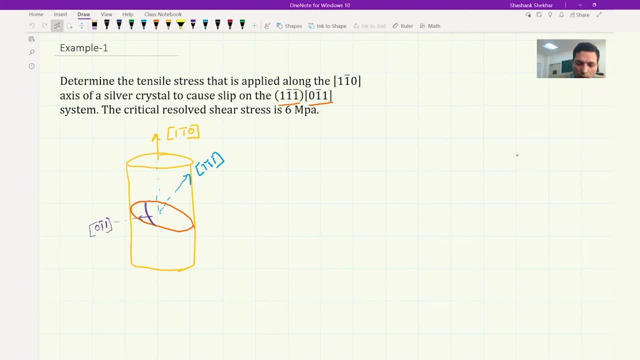 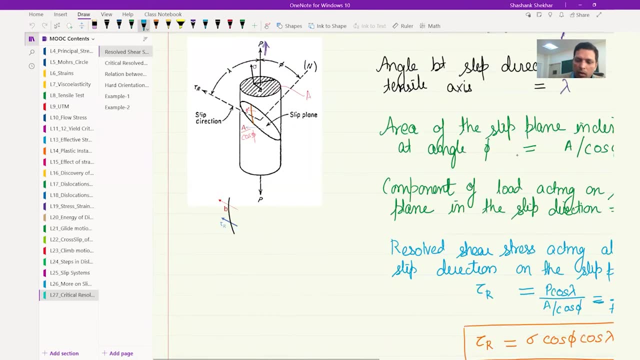 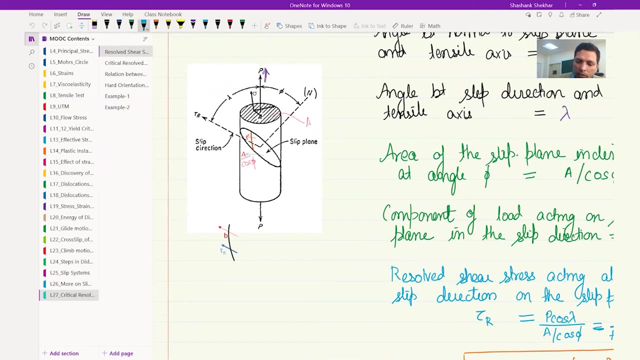 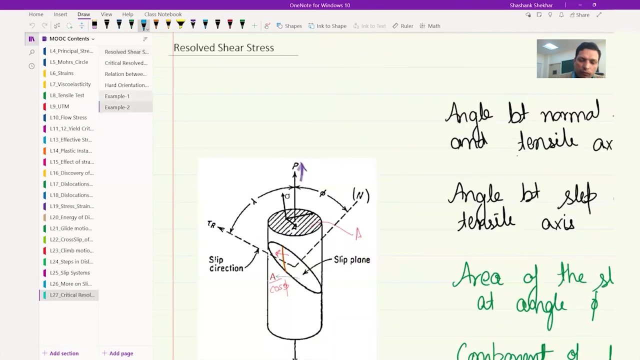 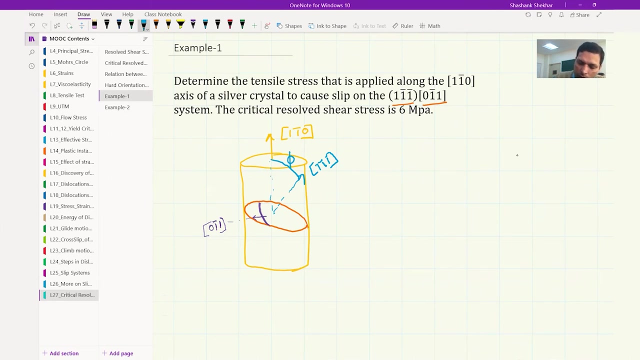 So we know that the angle between Berger vector and the normal is the phi and the angle between the normal, sorry angle, between the normal and the Berger vector, or the slip direction, is lambda and the normal and the loading direction is phi. So this is phi. 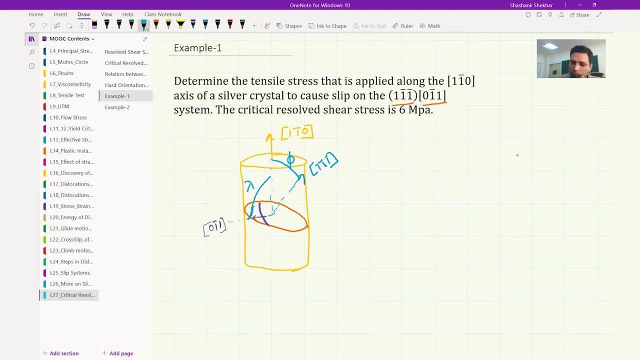 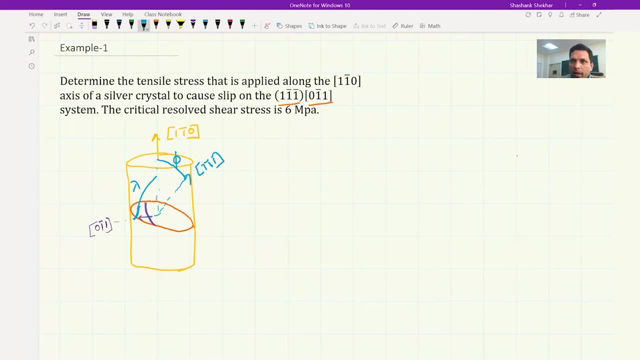 and this is lambda. So next, what we need to do is find the phi and lambda and therefore cos. phi is the, by taking the cos of these two vectors, and this is simple, that we have 1 into 1 plus minus 1 into minus 1 plus 0 into minus 1, and on the denominator, we will 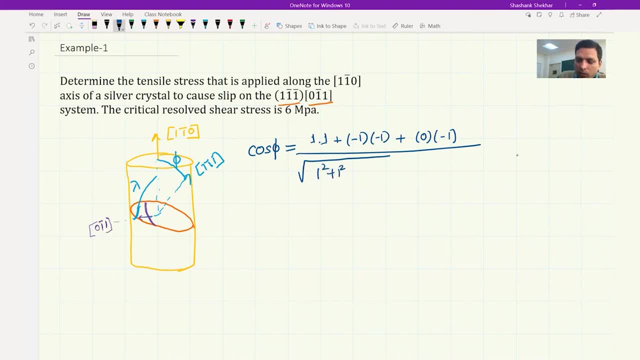 take the square root of this. So this is 1 square plus 1 square, actually minus 1 square plus 0 square, and the other one is minus 1 square. Sorry, this was just. we have not written it very neatly here It. 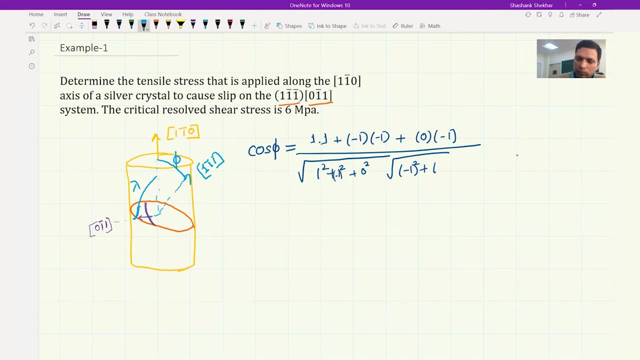 should just 1, there is no minus sign. So this is 1 square plus 1 square minus 1 square plus minus 1 square plus minus 1 square, and therefore it comes out to be 2 by root 2 into root 3, equal to 2 by root 6, and cos lambda will come out to. So now we are taking the 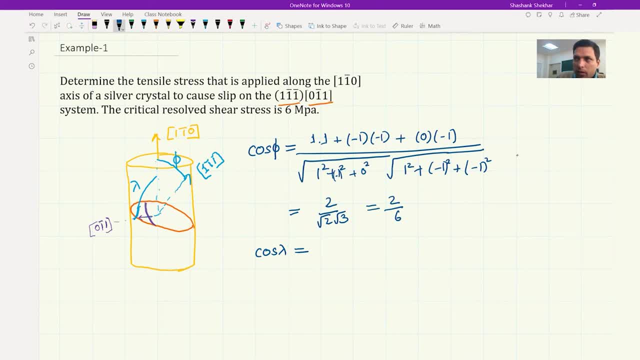 cos between 1 bar 1 0 and 0 bar 1, 1.. So this is 1 into 0 plus minus 1 into minus 1 plus 0 into minus 1.. And this one we already know is 1 square plus minus 1 square plus 0, and this one is: 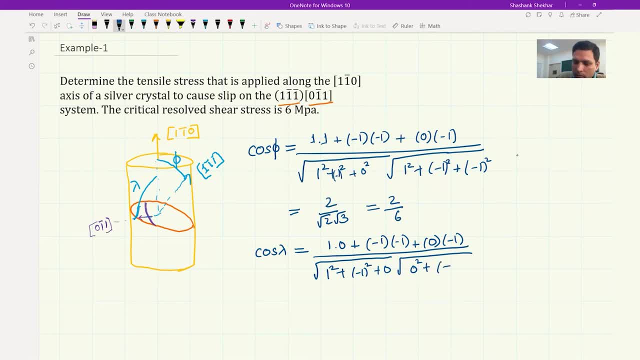 also the same 0 square plus minus 1 square plus minus 1.. Actually it is 0 bar 1, 1 square and therefore this is 1 over root 2 into root 2, equal to 1 by 2.. 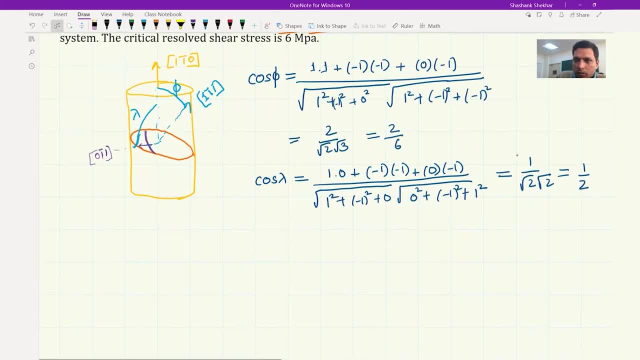 So we know that sigma is equal to 1.. Now CRSS: by assuming that this is the stress, normal stress, that will cause the dislocation to move, We have used CRSS and the CRSS is given to be 6 and therefore this is 6 by 2 by root. 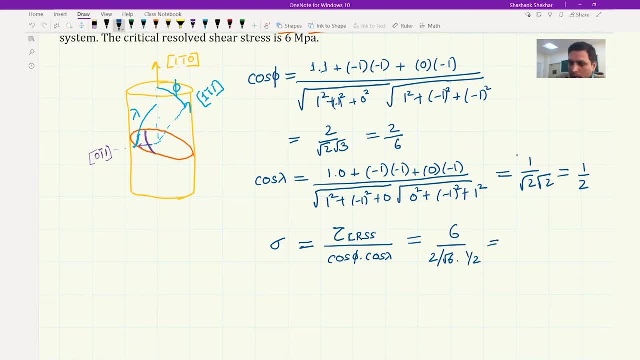 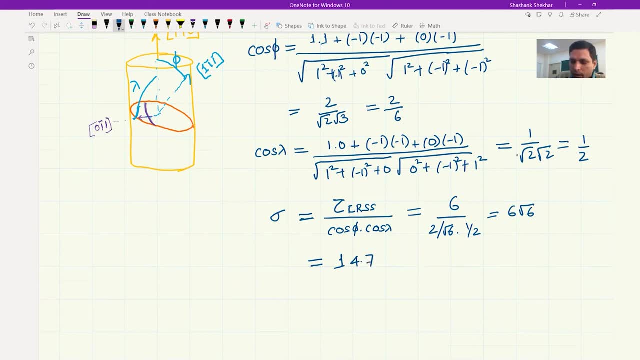 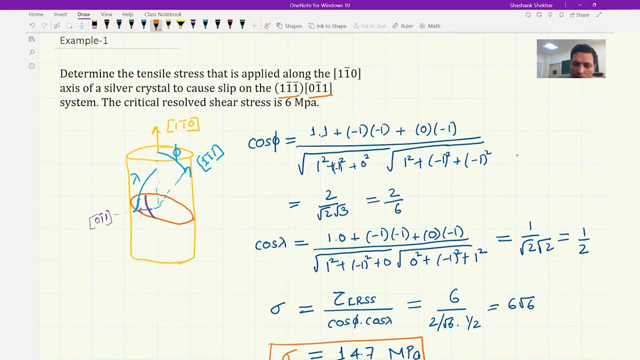 6 into 1 by 2 and this comes out to be 6 root 6 is equal to 14 by 2 by root 6.. So this is 14.7 megapascal. So if we have a dislocation with slip vector along this direction- and this is to be gliding- 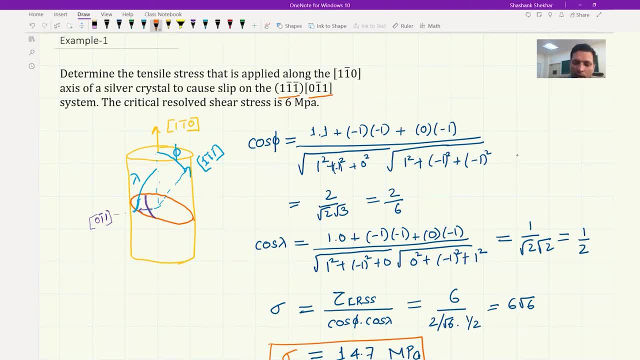 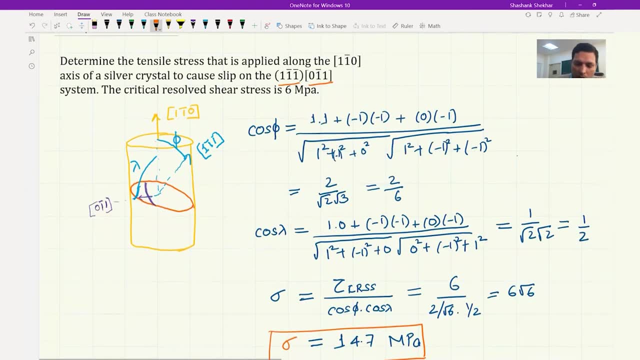 on 1 bar 1, 1 bar 1 bar 1, then you need to apply a normal stress of 14.7 megapascal along 1 bar 1, 0 for it to move the dislocation. Thank you. 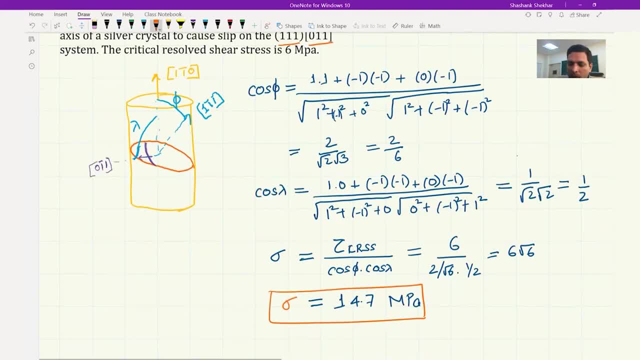 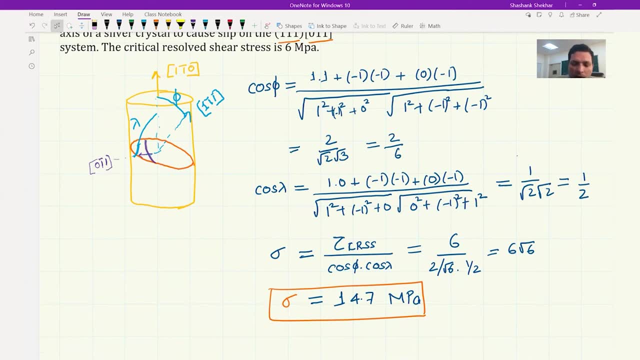 Thank you. That is what this example tells us, So you can see this is very helpful in helping us understand which particular dislocation would move and what is the stress required. Next we will look at an example to understand of the various slip planes in a system which one would get activated. 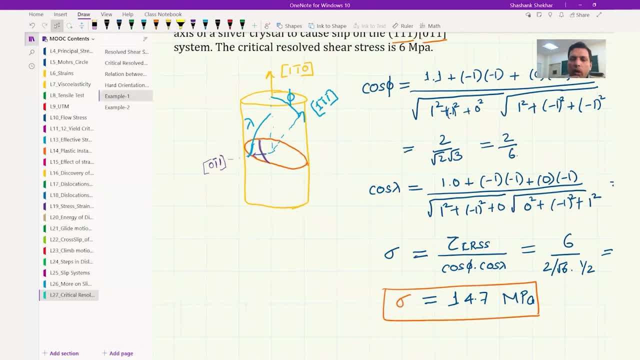 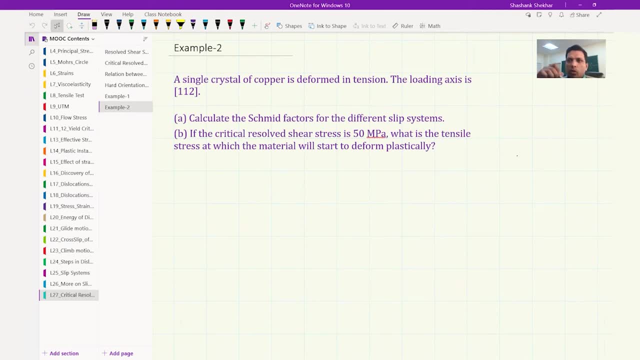 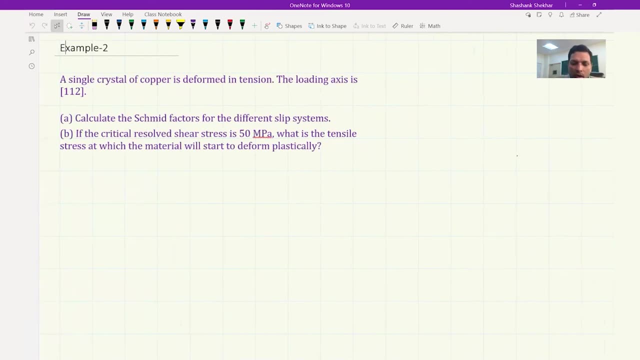 So here until now, in this example, we are looking at one specific slip plane, but the fact is that there can be more than. in fact, there is a lot more slip planes, as we will see. So you are in this example. you are given that a single crystal of copper is deformed in tension. 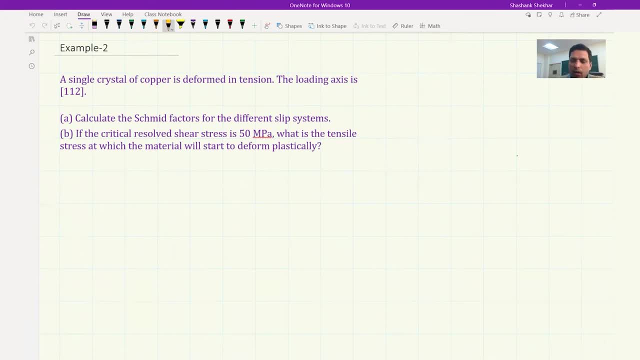 So again we are applying tension, and only that here it is in a little different direction. So this is again FCC and this direction is given as 112, and here you are not given any specific slip plane. You have been asked to calculate the Smith factor for all the possible slip systems, and for that we need to remember what are the possible slip systems in FCC. 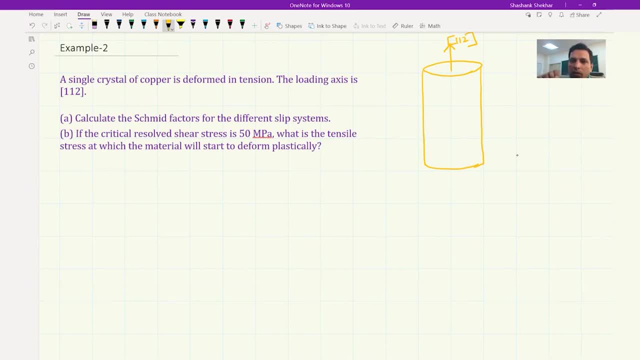 So 111 plane and 1110 type of directions, And you are also. the second part is, if you are also given, if the critical result, shear stress, is 50 megapascal, what is the tensile stress at which the material will start to deform plastically? 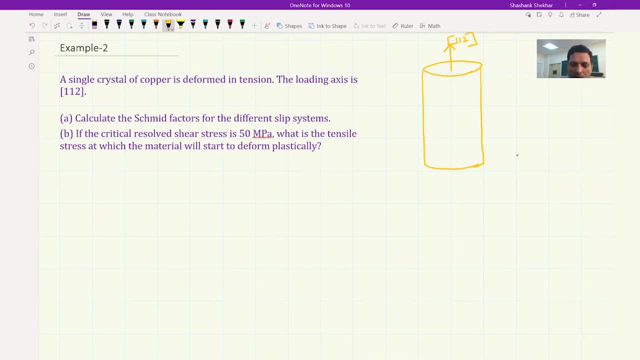 So first we will look at which one has the highest Smith factor and then for that we will calculate the tensile stress that would be required to make the dislocations move. So we will begin with the planes. So what are the possible slip planes? 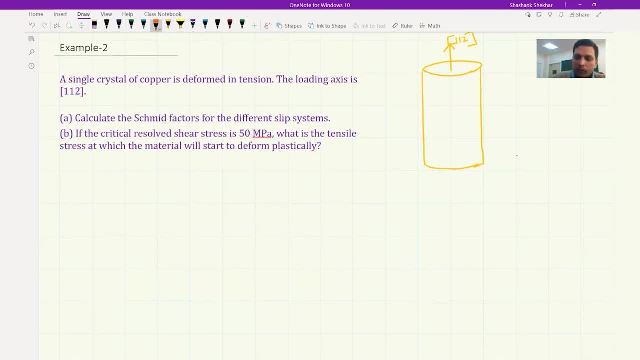 So you here, we can assume that basically there are slip planes like this: So here we have two planes, Here we have w, Here we have g Theatre Claro, And here we have k Here we have k Here, et cetera. And here we have a constant strike. Here is a negativeköhn 수 k. Here is a negativeköhn sagg, padreskønn患an sägn sug à näre. Here is a natives which, at least wheter, is positive. 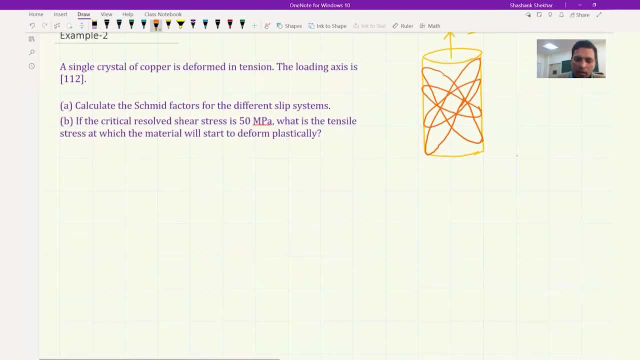 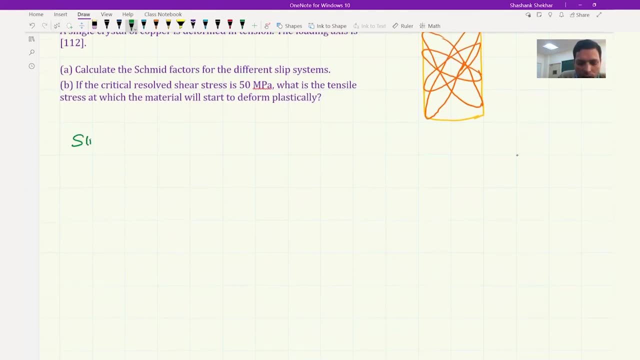 why i have been, i have drawn this. it will become clear to you like just in a moment. so what are the slip planes and the possible slip direction? so here we have the slip direction. so we will find cos phi, we will find cos lambda, and then we will. 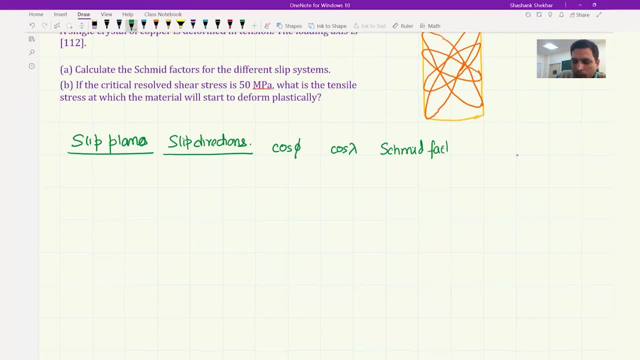 find smith factor and eventually we will find sigma. so this is the table and here we will use first the one one, one plane, and very easily you can show that directions possible for this are slip directions. I have written on the Burgess vector because we will have to add that factor of a by 2, but that is immaterial from the point of view of calculating. 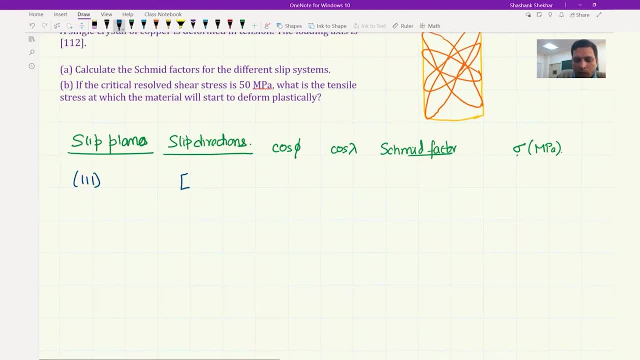 cos phi and cos lambda. So the possible directions are bar 1, 1, 0, or you can also take the negative bar 1, 0, 1 and 0 bar 1.. So I will show it for two systems and then I will just note down the values for other systems. 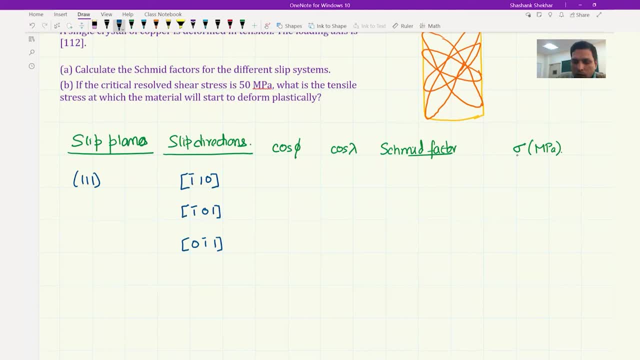 So over here we will take the cos phi, which will be between 1 1 1 and 1 1 2, and the number of vectorsY, and the number of vectorsY will be between 1 1 1 and 1 1 2.. 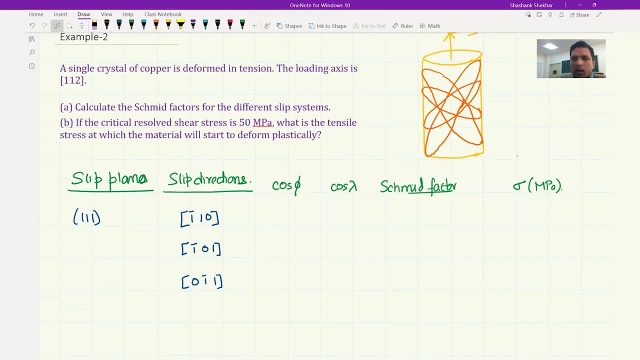 we know the relation cos phi equal to h1 k1, h1 h2 plus k1 k2 plus l1 l2 divided by h1 square plus k1 square plus l1 square. under root times. under root h2 square plus k2 square. 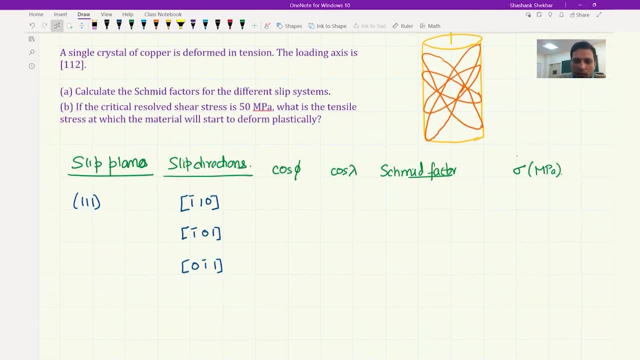 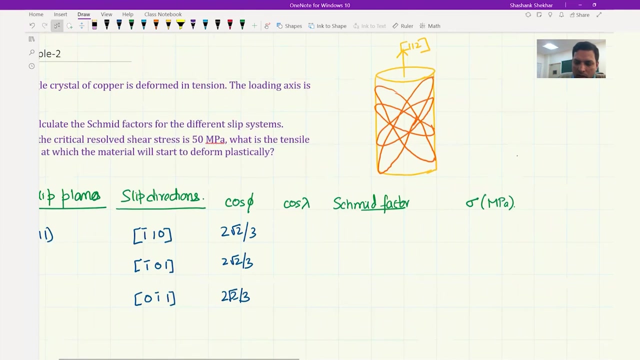 plus l2 square the one, the equation that we used in the previous example. so I will not go through that, but I will just write the values and it will be 2 root 2 by 3. this will be constant, because this is constant here and the cos lambda would be different. so you would see that 1 1 2 and bar 1 1 0. 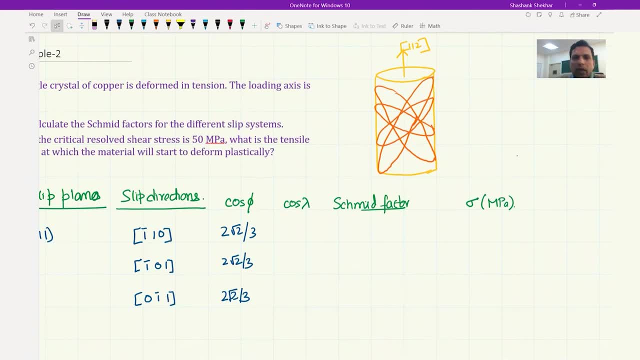 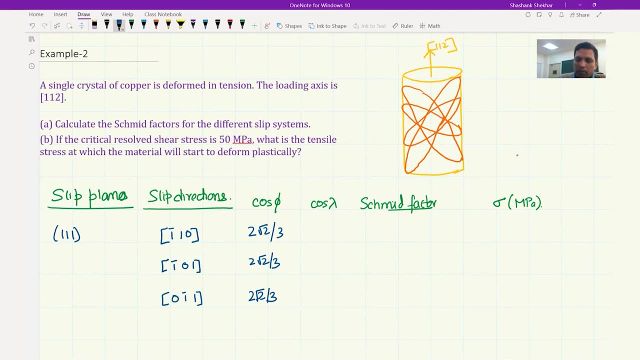 if you take the dot product then it is 0. what it means is that this slip direction lies in the same in the plane normal to 1 1, 2. so the bar 1 1, 0 is normal, is like this and which is normal. 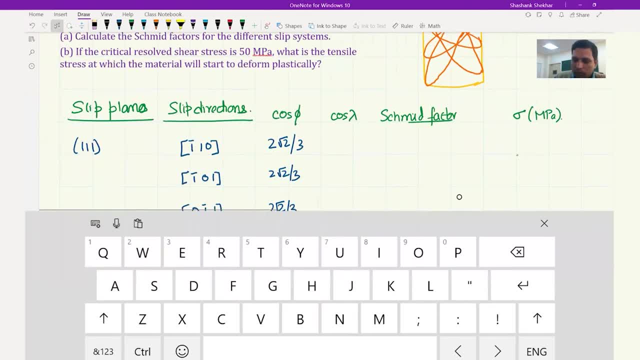 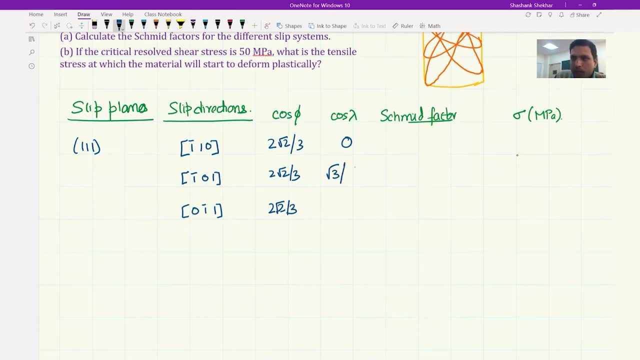 so that is not a good news in some sense. 0, and here we will get root 3 by 6, root 3 by 6. so again, I am not going through the equation. you would use the same equation that we used in the previous example and you can find cos phi. 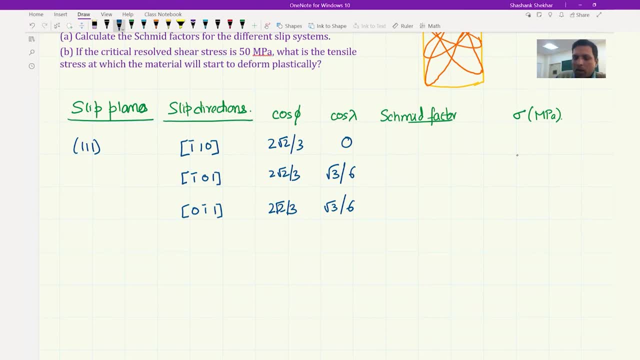 and similarly, you have found cos lambda and then you take the product to find smith factor. so this is 0, 1, 2 and 1: 2, so this is 0. this is root 6 by 9. this is root 6 by 9. 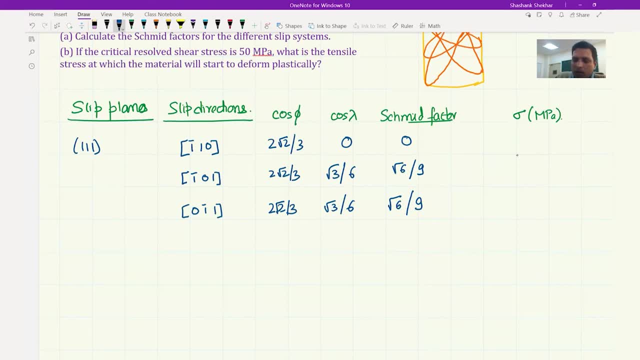 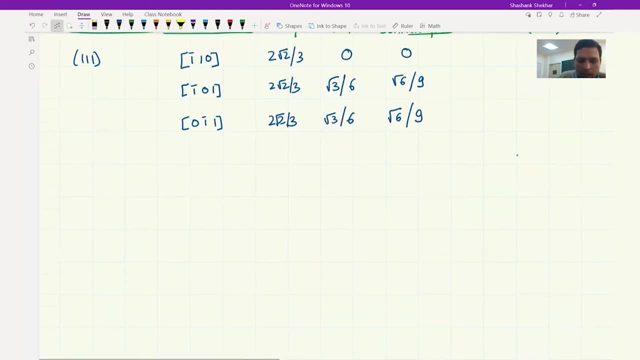 I am not finding the sigma values. I will do it only for the 1, which comes out to be the lowest. next plane that we will select is so there are four 111 type planes, and so we will need to do this 4 times, and the directions here are 117 and 218, one and one times here, and 219 or 218, one and anotherHuh. so, thehyun, some analysis field is not there by working on the Supra. so, in sum, try to review if there is some actual variation. is there is not everything? okay, so that I know the numbers we have in the set数. but we will work out here most of all alone. left letter, we can right and right order. we see that node value. we are saying 4線, let's dialogue here, and so we will� 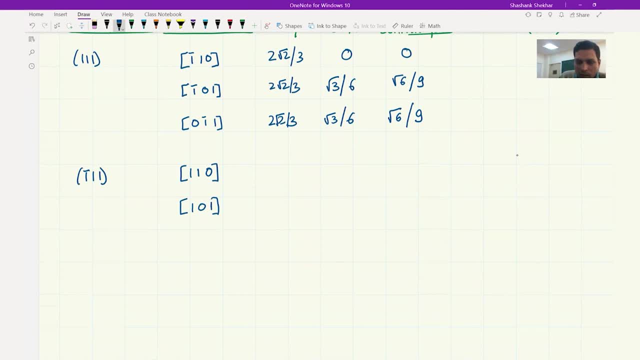 0, 1, 0, 1 and 0, 1, 1.. So you can see that these two are dot. product is 0.. So this is indeed the vector that lies on this plane, and then we will calculate the cos phi which would again become, which comes out to same value, and the cos lambda comes out to. 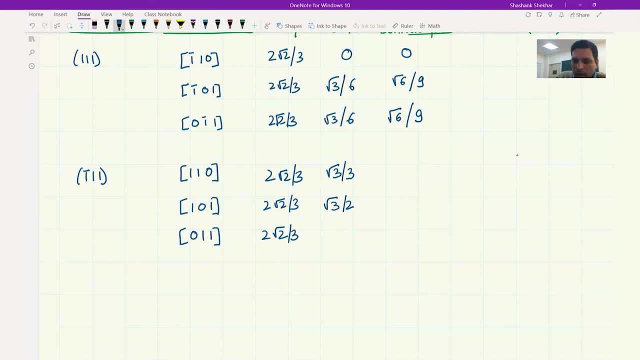 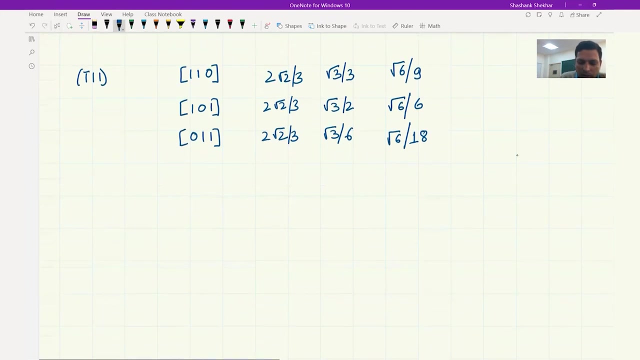 root 3 by 3, root 3 by 2 and root 3 by 6.. So the overall smith factor comes out to root 6 by 18, and the third plane we will select is 1 bar 1, 1 and the 3. 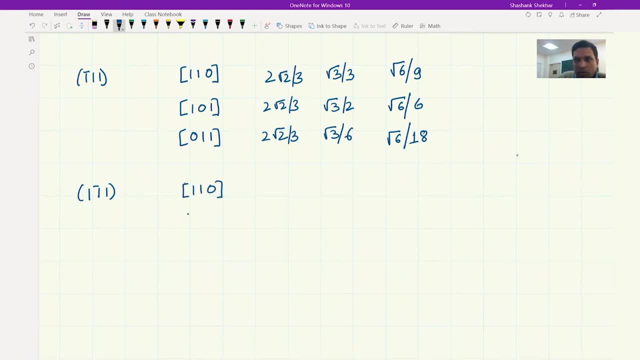 directions are: 1 1 0, bar 1 0 1 and 0 1 1 and here also the. this is a little different, okay, so I have made a mistake here, that's there is no 2 here actually, so this one is also root 2 by 3. 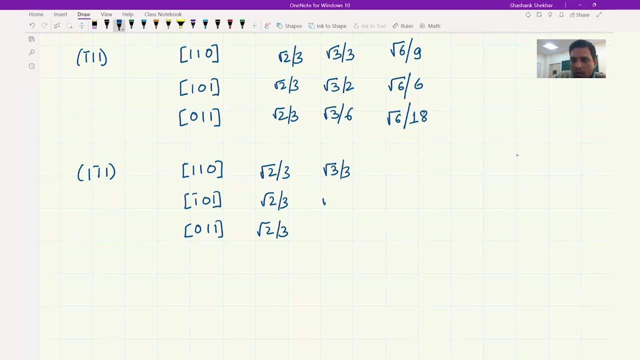 and the values are: root 3 by 3, root 3 by 6, root 3 by 2, and the smith factors come out to root 6 by 9, root 6 by 18, root 6 by 6.. So we have done for three planes. now the fourth one is a little bit. 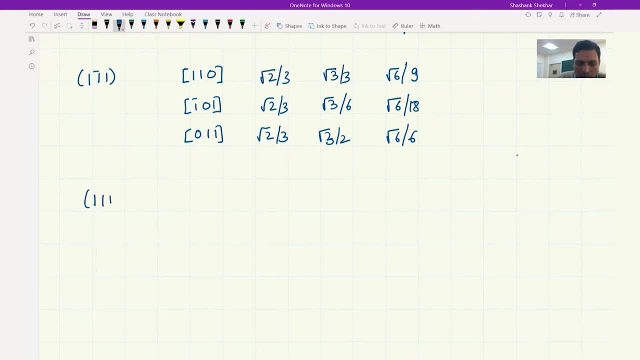 you can say very different: 1, 1 bar 1, and the four directions are bar 1, 1, 0. now what happens here is that 1, 1 bar 1 is at 90 degrees, so the cos phi comes out to be 0.. 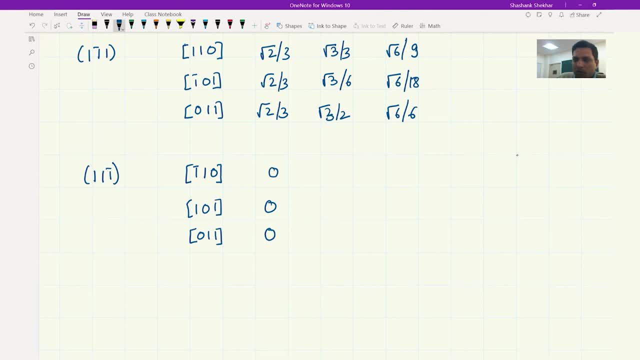 So now, from here itself, we can say that the m would be 0, but anyways, we'll go through the motion and find out the values. so these are the lowest smith factor- and certainly we are not interested in this, which is the highest smith factor that we see over here, and you would see that this value is 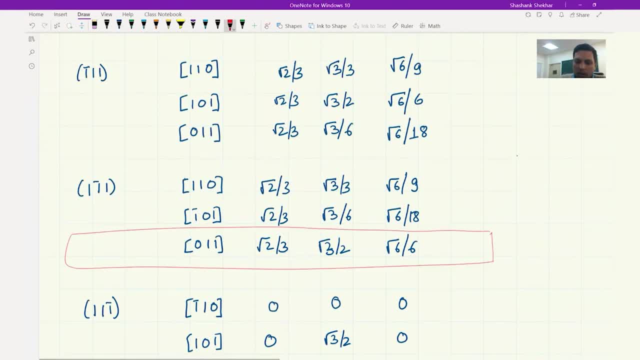 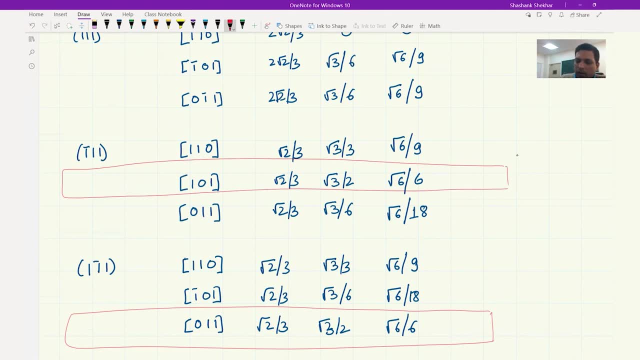 highest. similarly, we get another root, 6 by 6.. which is this? so these are the slip systems where the smith values highest and which would mean that the yield strength value would be lowest, and if you calculate, what you would see is that 122 mega pascal. 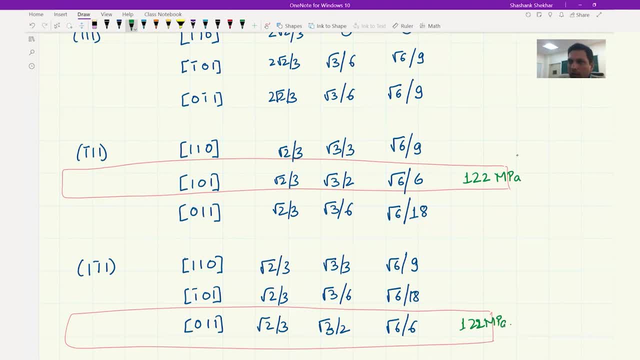 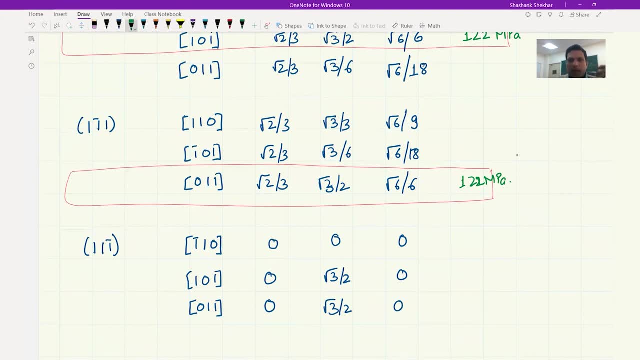 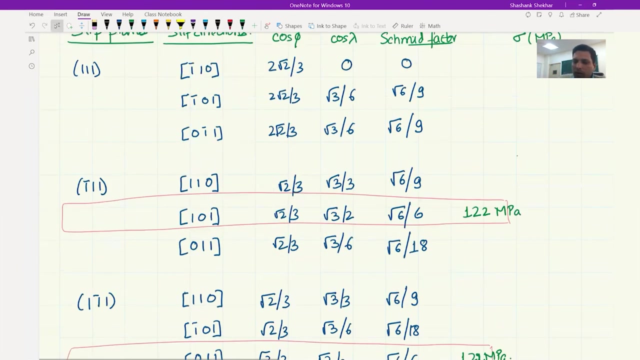 122 mega pascal, and just so. what this means is that if this is a 0, no matter how much stress you apply, this will not deform. so this will. i will just say nd, meaning not deformed, and the nd similarly we had obtained was 0 over here, so this is also non-deformable plane. 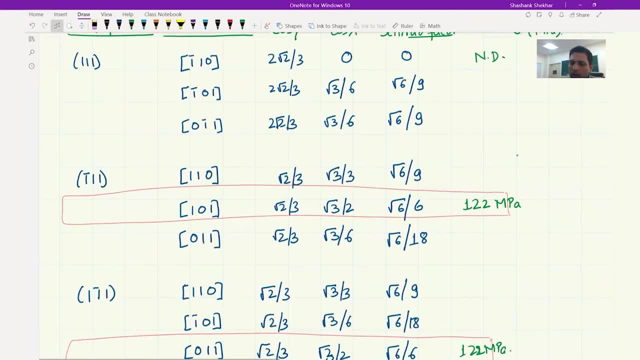 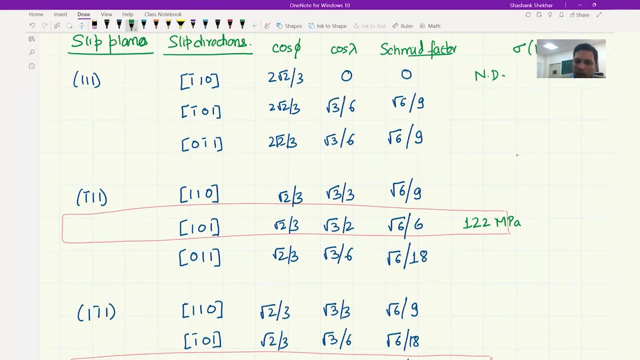 or system. so this one is non-deformable. and just for the sake of completion, it was not. it is not required here, but just because we are here i will. for the sake of comparison, i will put the values of how much stress would be required for dislocation to move in this slip system. you would see that it will come out to 184. 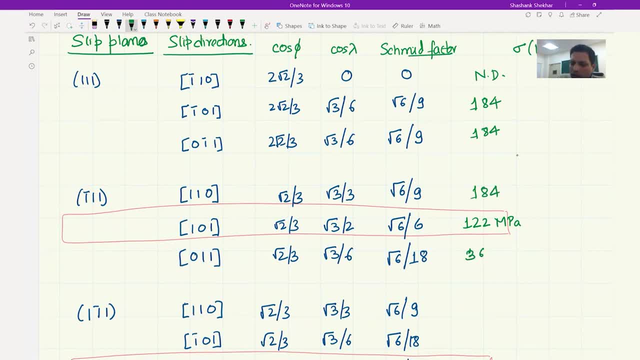 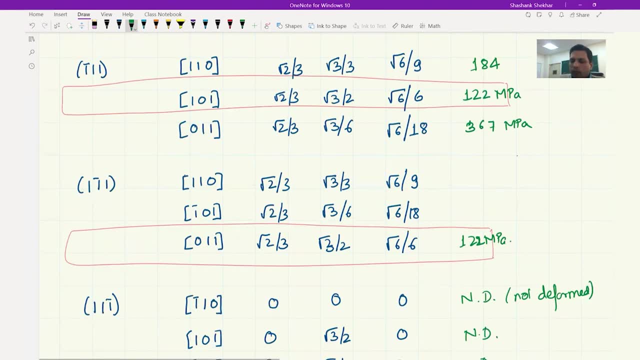 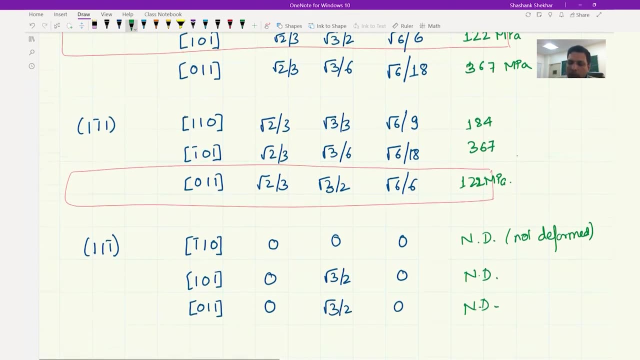 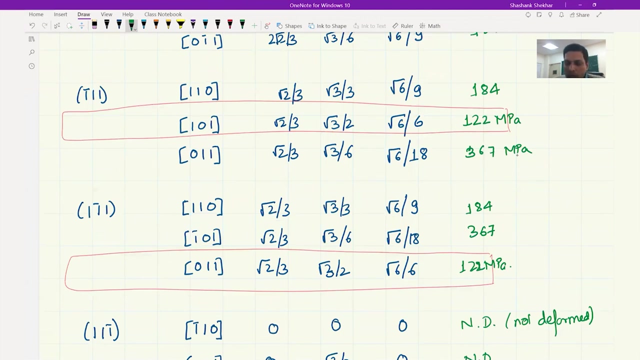 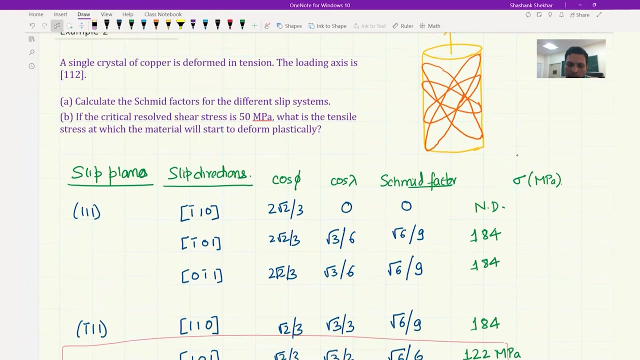 184, and this one will be. this mid factor value is very low: 184, 367. so these two have the lowest amount of tensile stress required for dislocations to move. so for this particular orientation we have four different planes and we on the four different planes we have again three different directions. 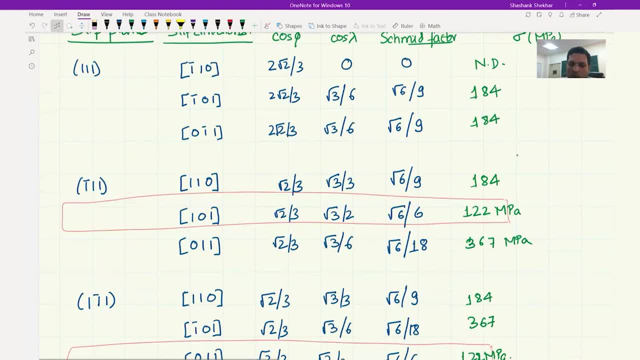 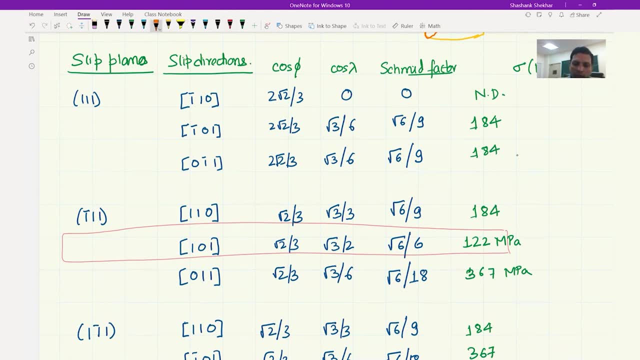 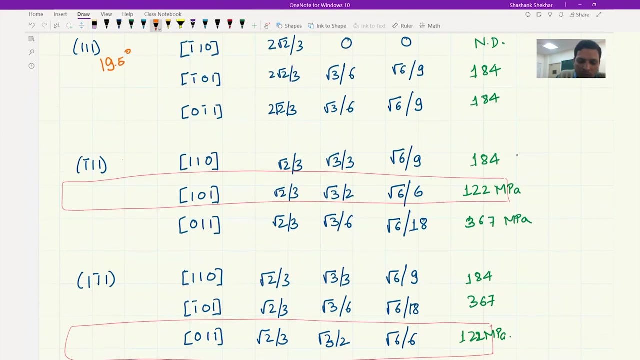 and for that we get these different values now for again. uh, what is what would be useful here if i put in the values in terms of orientation, rotation or the angle between this 111 plane and the tensile direction, so what you would see is this one would come out to 19.5 degree. this one will come out to 61.8 degrees. this one is also. 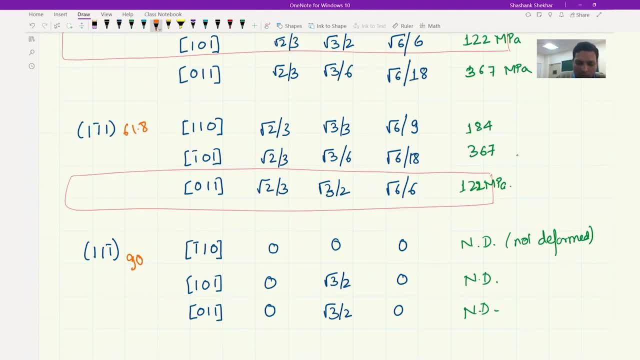 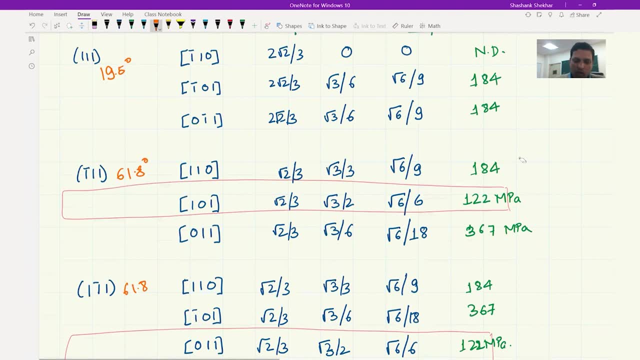 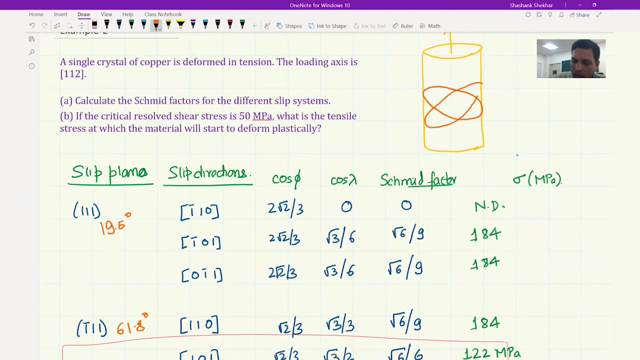 coming out to 61.8 degrees and this is coming out to be 90.0 degrees and this is coming out to be 90.0 degrees. so actually the way i had drawn is a little bit incorrect. so there are two planes which are at 61.8 degrees, so something like this and something like this. on the other hand, we have 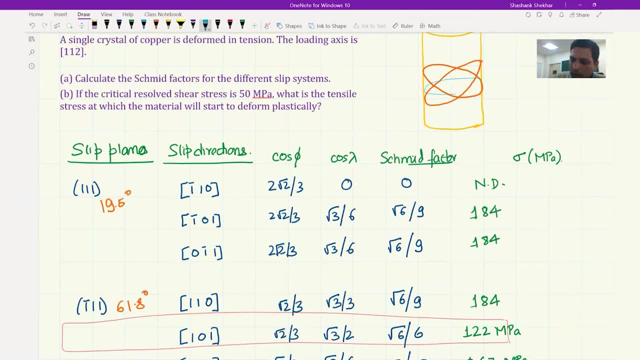 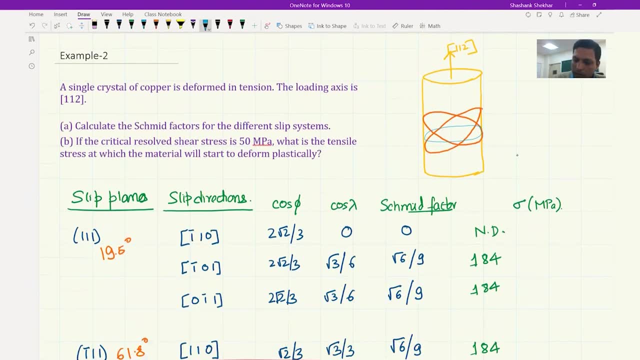 a plane at 90 degrees, so it is like this, and one is at 19.5 degrees, so this one is at 90 degrees. so, clearly, the stress is required for this plane and for this plane. in fact, this one is undeformable. this is the last one where the 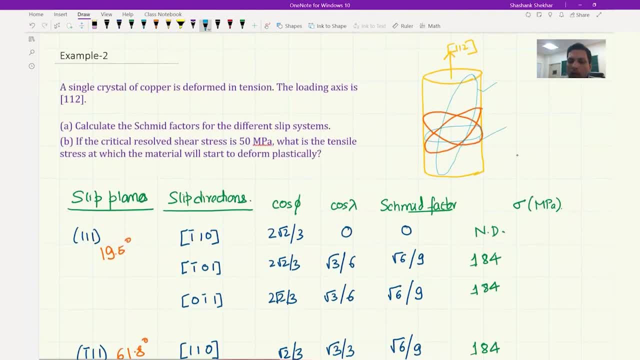 schmidt factors come out to be zero, meaning no component of load will lie in here, which is what we know- and therefore there's no amount of stress can make the dislocations move in this plane. here, this one, you can make it move, only that you would need much higher stresses, and which? 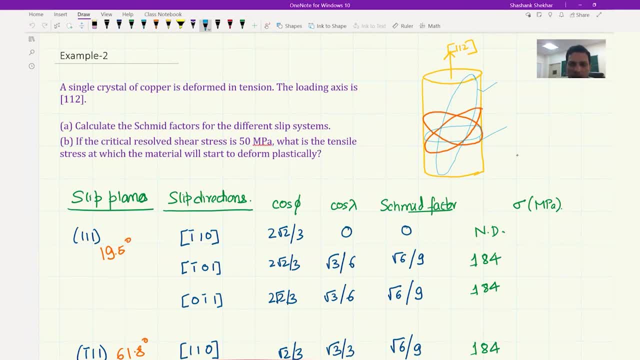 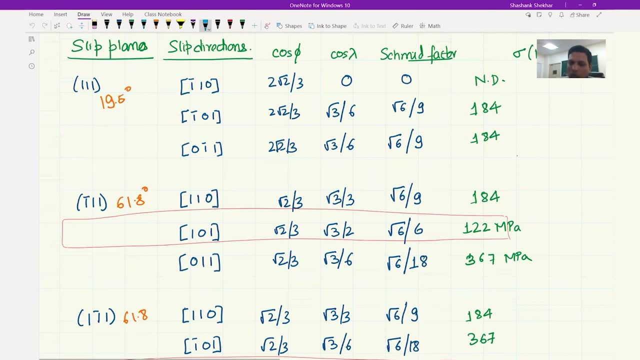 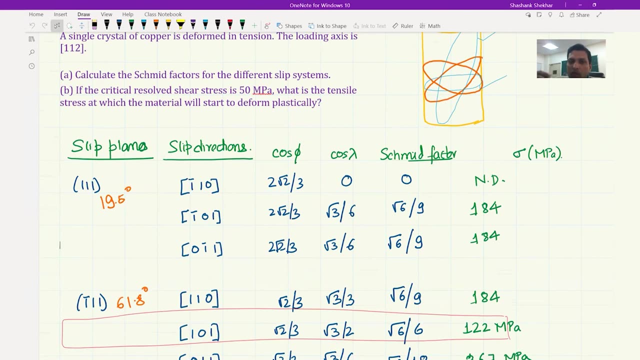 is clear over here, and in fact one of them still would be non-deformable for these two systems. we see that we do get. these are close to 45 degrees, which is what we expect, which is where the shear stresses would be highest. but then we also have to look at the direction. 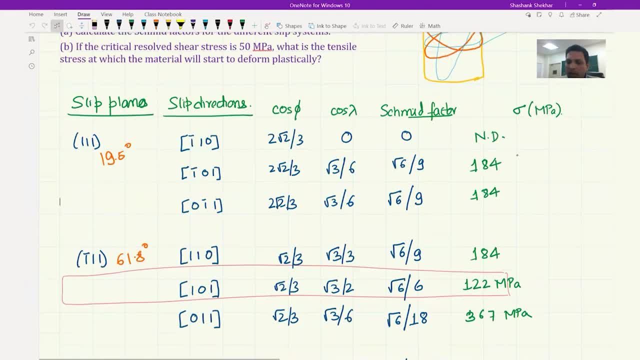 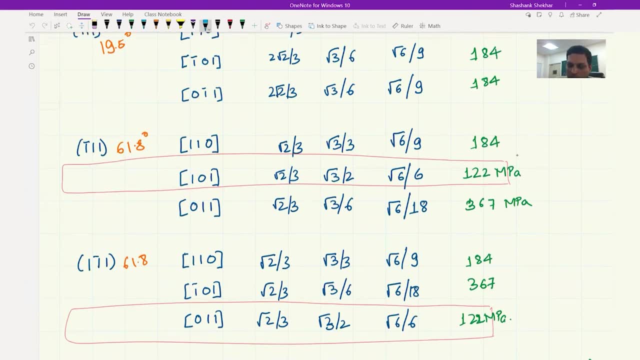 and looking at the direction, we can clearly see that there are two, one direction in this, one bar one, one one plane and one bar one, one plane where the yield stress required for moving the dislocation is lowest. so these are our preferred- or you can say- and orientations that we are looking for where the